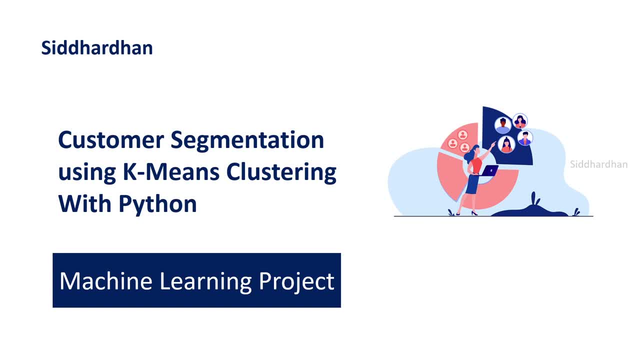 Hello everyone, I am Siddharthan. This is the 13th project video in our machine learning project series and in this video I am going to show you how we can use k-means clustering algorithm to do customer segmentation. In customer segmentation, we will try to group customers based on their 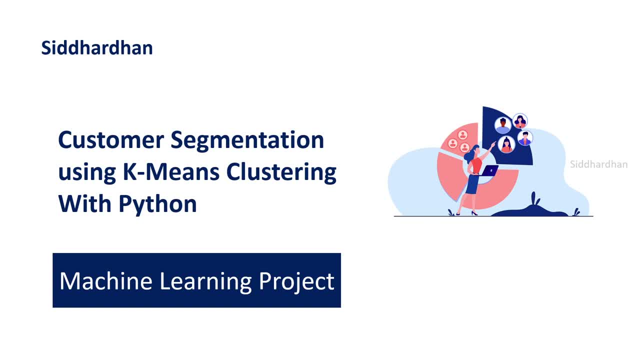 spending patterns and purchase behavior and such kind of things. okay, So this is what we are going to achieve in today's video. So, in case you are watching my videos for the first time, hi, In this channel I am making a project based machine learning course and you can go to the playlist. 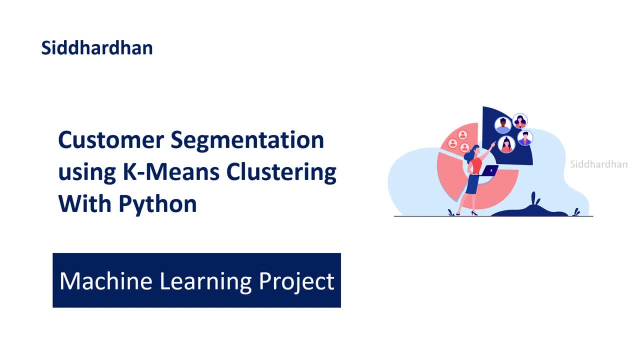 section to learn about my other machine learning project videos and also about my machine learning course. okay, So, with that being said, let's first try to understand today's problem statement, After that I'll explain you the workflow which we are going to follow, and after that we can. 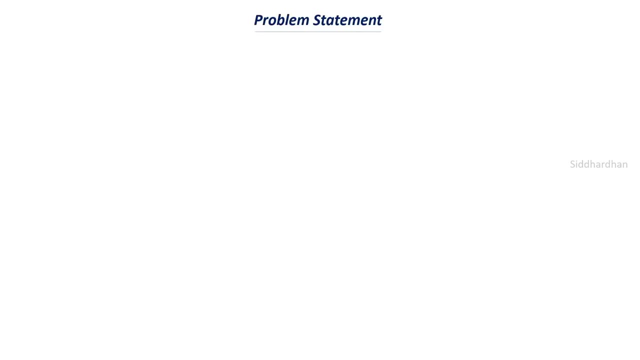 get started with coding part, okay. So this is the problem statement. Consider that there is a very famous mall and you are a very experienced data scientist and this mall wants to get insights about their customers and they have their customer data regarding their purchase behaviors and other aspects to it- okay. So as a data scientist, you can build a system that 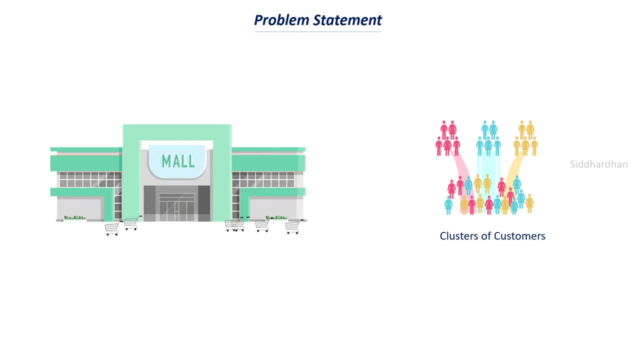 can cluster customers into different groups. So one group of customer may represent those that tend to purchase more in that mall and some other group may represent a group of customers that don't purchase that much in a mall. So you know, having these groups of customers will give us better. 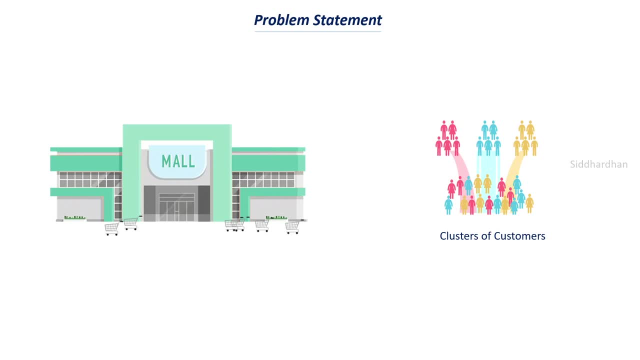 insights and it helps that. it helps that mall to make better business decisions, to make better marketing strategies and such kind of things. So this is the problem statement which we have today. So this is an example for clustering machine learning projects or clustering machine learning problems. So so far we have discussed about only the classification and regression. 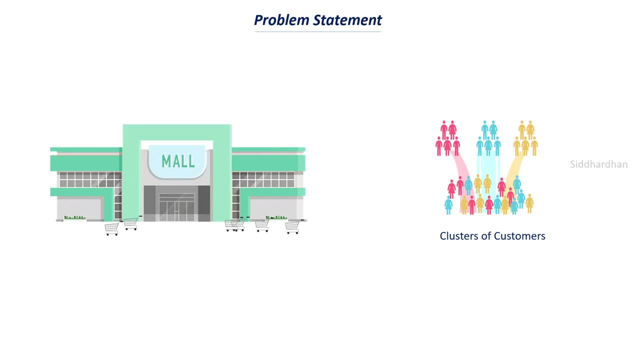 problem. So classification and regression comes under supervised learning, whereas this clustering comes under unsupervised learning. So we have already made videos regarding these topics. so if you are not you know clear about those classification, regression or clustering, just let me know in the comments. I'll give the link for those. 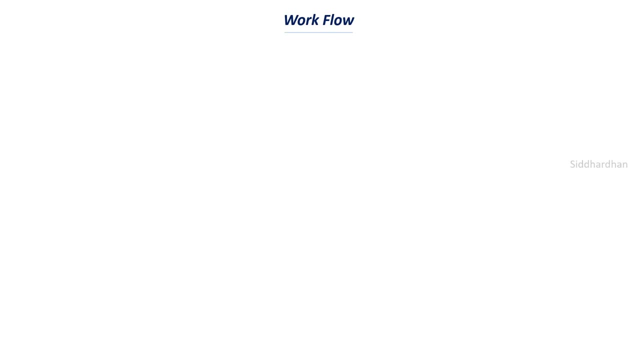 videos. okay, So now let's try to understand the workflow which we are going to follow. First, we need this mall's customer data, because we need data to train our machine learning models, right? So first is getting this customer data and once we have this data, we need to process. 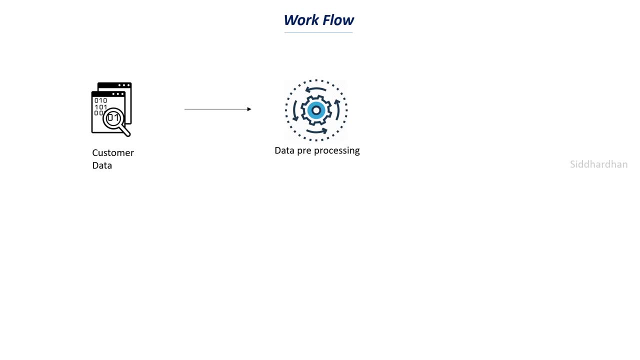 this data So we cannot feed this data directly to our machine learning model. So we need to select few features which we need, So those things will be covered in data pre-processing. Then we need to also analyze the data So to see which features are important for us. 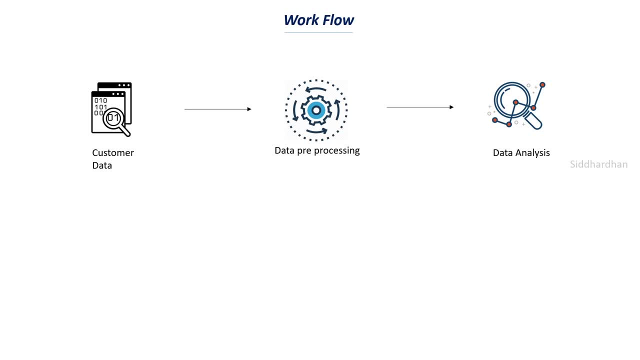 What are the various features that particular data set contains and such kind of things. So that will be covered in data analysis, and after that we need to choose the correct number of clusters. So we need to, you know, tell the machine learning model that I want three clusters. 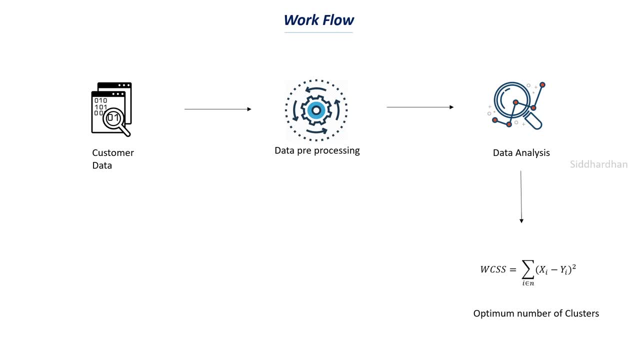 or five clusters, or you know this many group of customers. I want to split my data into these many groups. So we find that number by using a method called as within cluster sum of squares. So we will try to find this WCSS value and we, you know it tells us the. 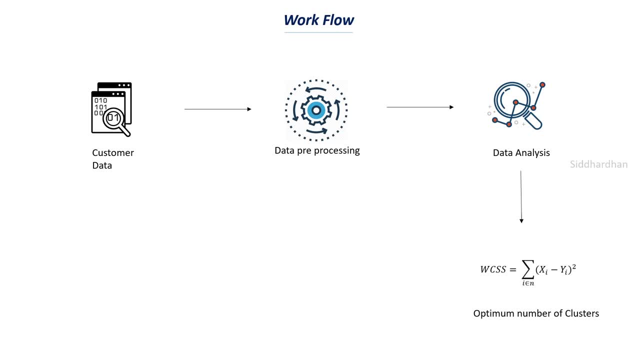 correct number of clusters that is, you know, suitable for this particular data set. So I will explain you more about this. when we implement this method and once we have the number of clusters we need, we can feed this data to a k-means clustering algorithm. So once you feed this algorithm to this, 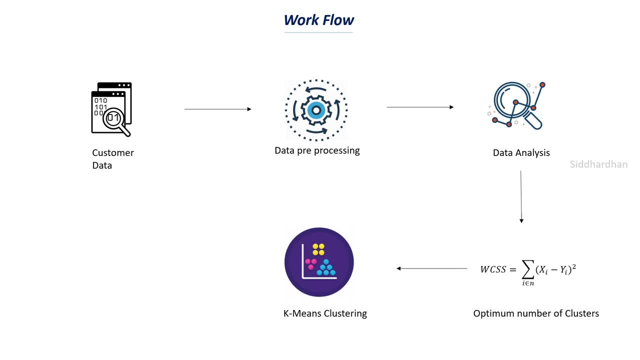 model. it can group the data depending on the similarities, depending on the similar spending pattern, etc. okay, So after that we can visualize these clusters by putting these data or the predictions made by this particular k-means clustering model into plots to get better insights about this data. So this is 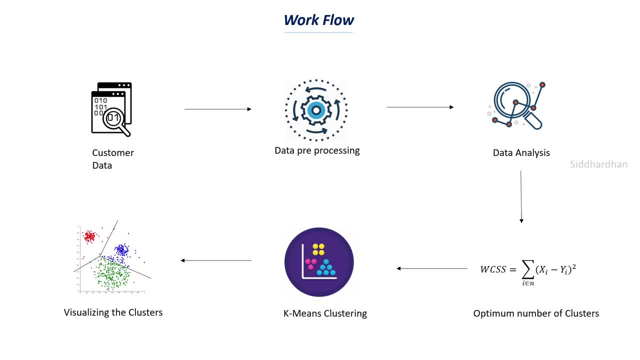 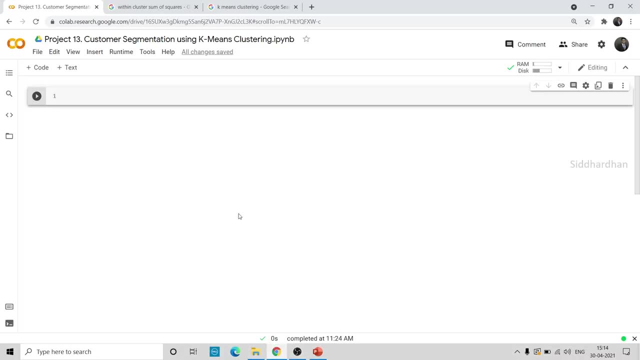 the workflow which we are going to follow. okay, So now let us get started with coding part. So I will be doing this programming in python, and for python programming I am going to use google collaboratory. I will link the video for this google collaboratory. I have already. 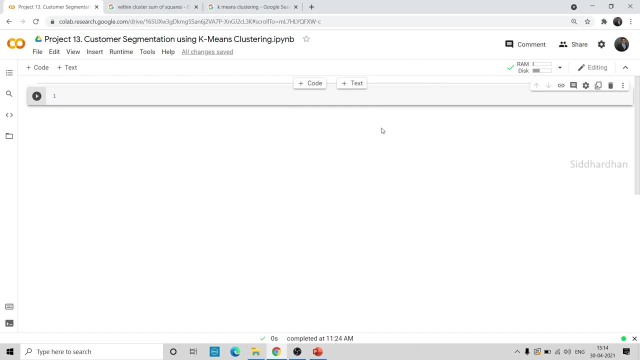 made a video explaining all the features of google collaboratory and how you can access google collaboratory. I will given the cards for the link of that video. So if you are not aware about this google collaboratory, you can watch that video, okay. So, with that being said, 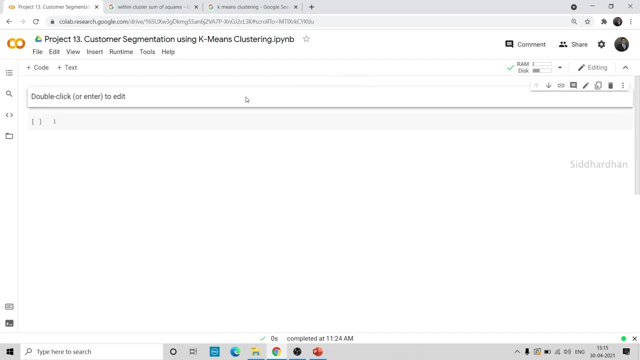 now the first step which we need to do is import the dependencies, So I will make a text here as importing the dependencies. okay, So dependencies are nothing but the libraries and the functions which we will use for this particular project. okay, So I will import some basic python libraries. 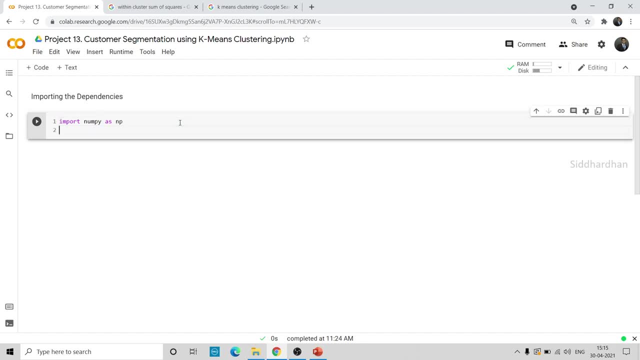 numpy and pandas. So import numpy as np, and let us also import pandas as pd, and import matlibpyplot as plt and import seaborn as sns. and finally, I will import sklearncluster. okay, So it should be from sklearncluster. okay, So from sklearncluster. 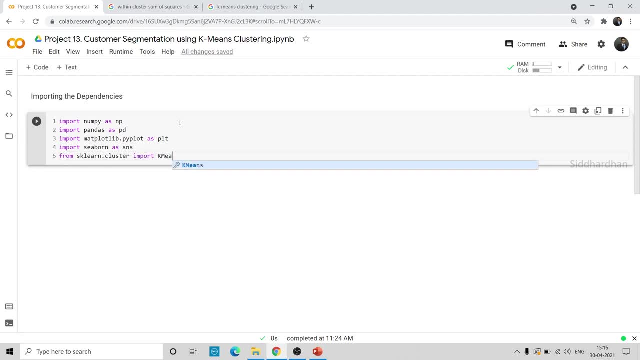 import kmeans. Okay, so these are the dependencies which we need. So numpy is all about numpy arrays, so this numpy library is useful for making numpy arrays. and pandas is all about making data frames. So data frames are nothing but structured table, So the data set which we have is in in the form of. 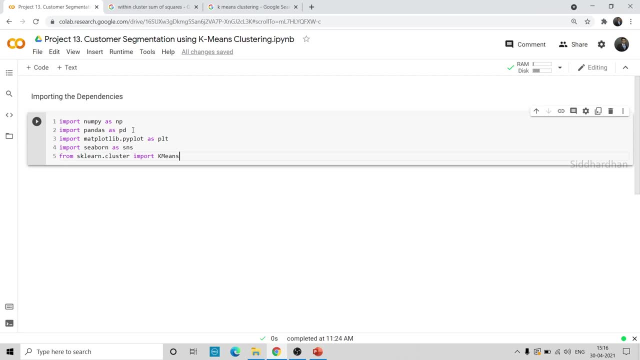 a csv file. csv represents comma separated values, So it is better to load the data into pandas data frame, as they are, you know, structured tables, and we can do better processing and analysis. and then we have this matplotlib library and a seaborn library, and these libraries 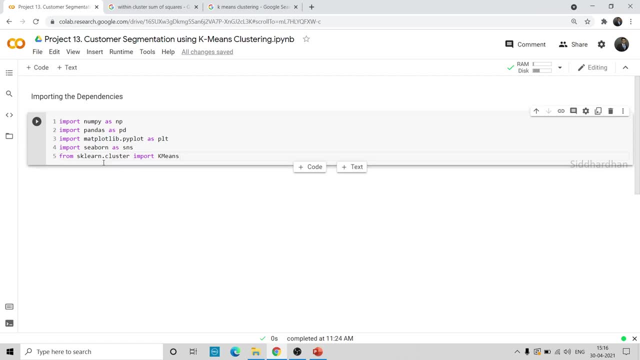 are useful for making plots, so these are data visualization libraries. and finally, from sklearn, from this sklearn library, in this cluster module, we are importing k-means. so this is the k-means clustering algorithm. okay, so these are the dependencies which we need, so let's run. 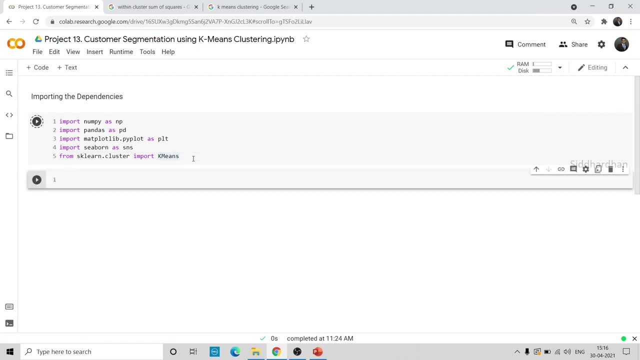 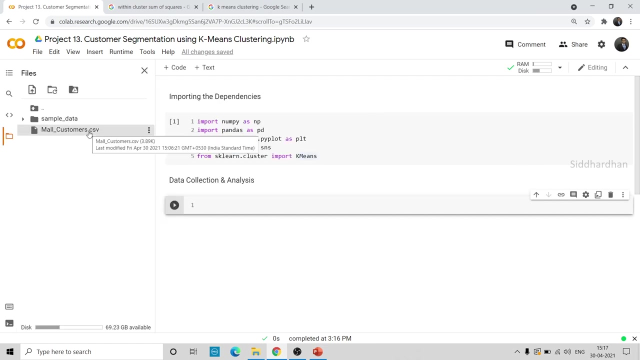 this cell. to run this cell and go to the next one, you can press shift plus enter. okay, so the next step is about data collection and analysis. okay, so you can see this files option here. right, so go to this files. so, as you can see here, i have already uploaded my data set file, so i give the. 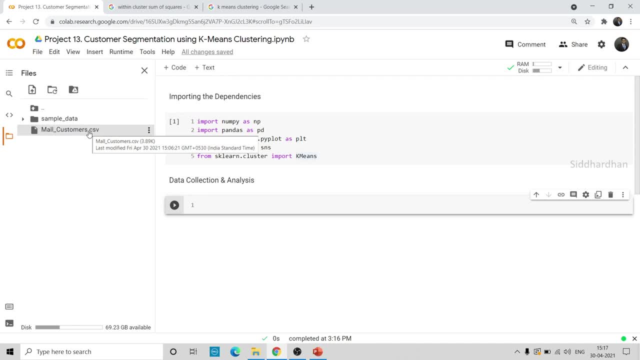 link for this data set file in the description of this video so you can download it. and from here you can also find this data set in Kaggle. just search as mall customers, data set Kaggle, so you can find this data set. so after that, so once you open this files, you can go to. 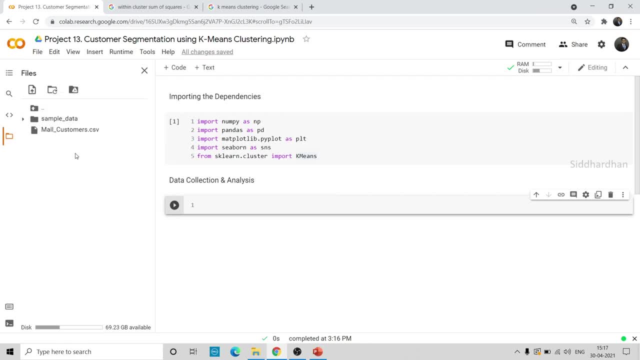 this upload to session storage option. from there you can upload your data set file. now i will copy this path of this particular file. so once you give this options, you will find this copy path. so i'll copy the path of this file. now we need to load the data from a csv file so you can see that it is in. 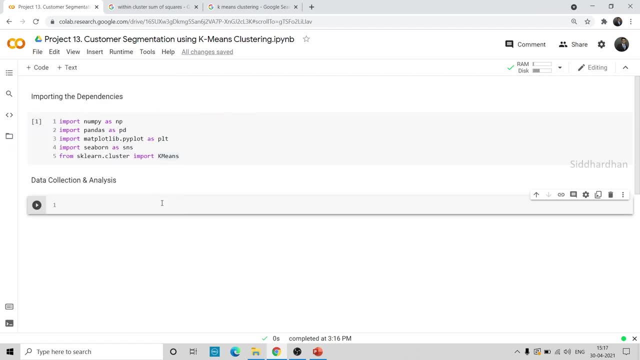 a csv file right now let's load it to a pandas data frame. so i'll make a text here as loading the data from csp file to a pandas data frame. okay, so let's name this data frame as customer data. so customer data is equal to. so we have imported pandas in the short form in the updated form as: 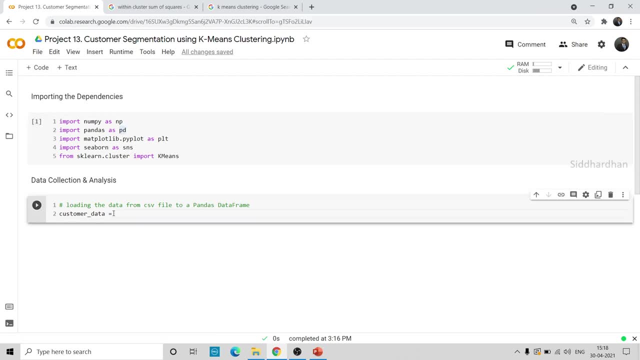 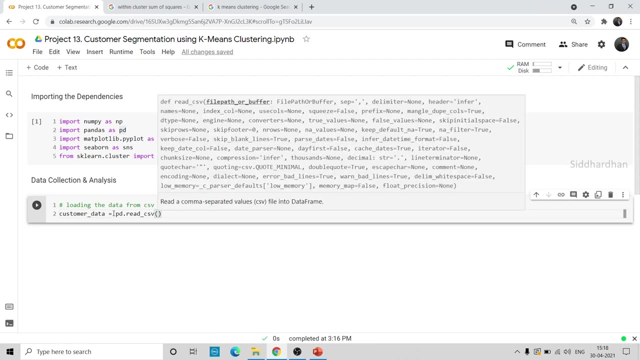 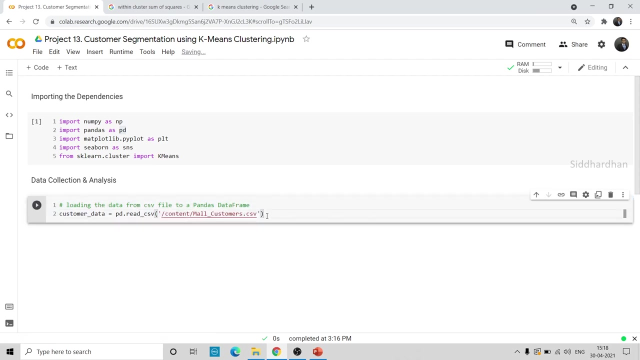 pd right. so we need to mention pd. so pd dot. read csv. so this read csv function will read the csv file and load all the contents of the csv file to a pandas data frame. so inside this we need to mention the path of the file. so we have already copied the path of the file, right, so now let's. 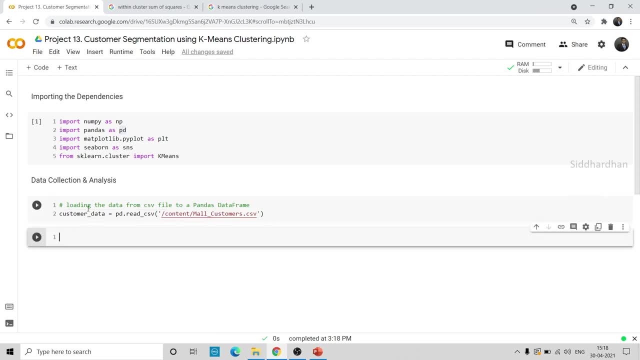 run this. so this will load this to the data frame named as customer data. now let's try to print the first five rows of this data frame and see what are the columns or what are the features we have in this data set. so first five rows in the data frame: 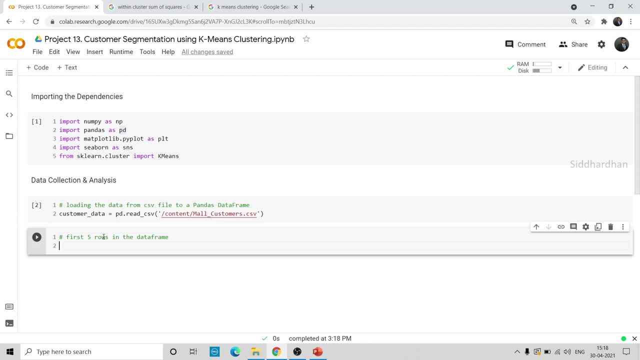 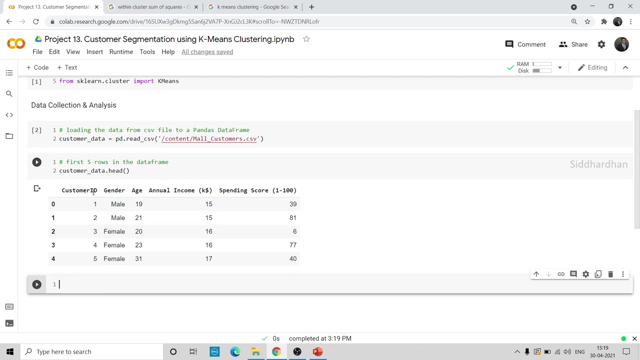 okay, so let's mention the data frame, which is customer data dot yet. so this yet function will print the first five rows of the data frame. okay, so, as you can see, here we have first five rows and totally we have about five columns. the first column is customer id, so each customer has a unique. 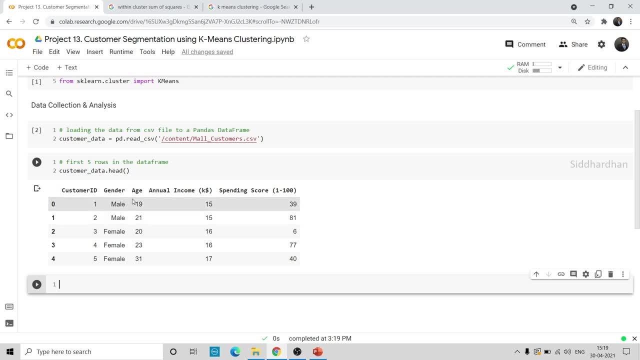 id and we have the gender of each customer and we also have their age and their annual income in thousand dollars. so fifteen represents fifteen thousand dollars. seventeen represents seventeen thousand dollar annual income. okay, and finally, we have spending score and the value of spending scores range from one to hundred if the 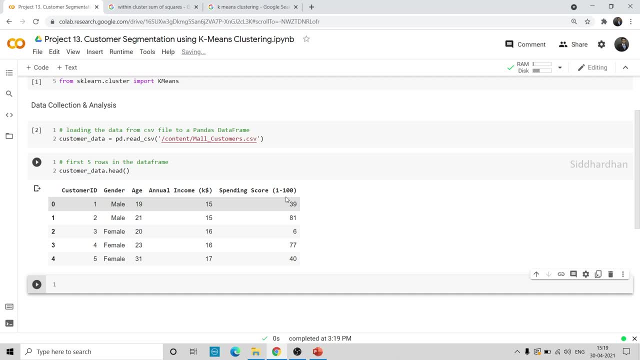 value is, you know, greater than seventy, and if it is close to under, that means that person is buying so much in that particular mall. there, i mean, they are spending more, and if the value is kind of less, that means that person is not spending that much in that particular mall. okay, so this is all about. 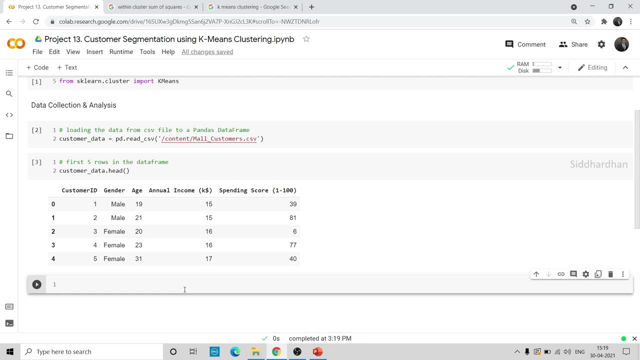 this spending score. now let's try to find how many rows and columns we have in this particular data frame. okay, so we already see that we totally have six columns, right, so finding the number of rows and columns? okay, so i'll mention the data frame name: customer data dot shape. let's run this. 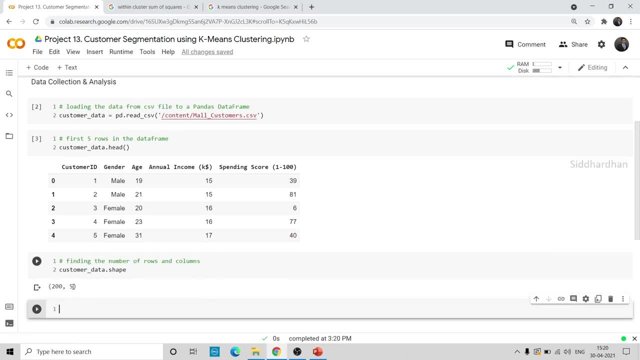 so the first value represents the number of rows and the second value represents the number of columns. so 200 means so totally we have 200 rows or 200 data points. that means we have the data for 200 different customers. so this is a good sample size, and totally for features or for columns. so 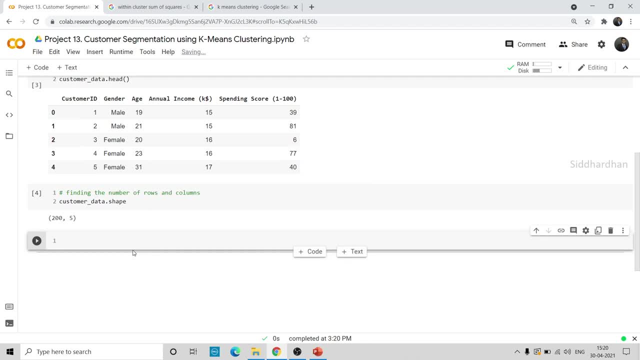 we have totally five columns right, so this is, uh, the shape of this data set. now you can get some more information about this data set using dot info function. so these are the some basic things we used to do in all the projects we do. so it is you know better to understand our data before. so 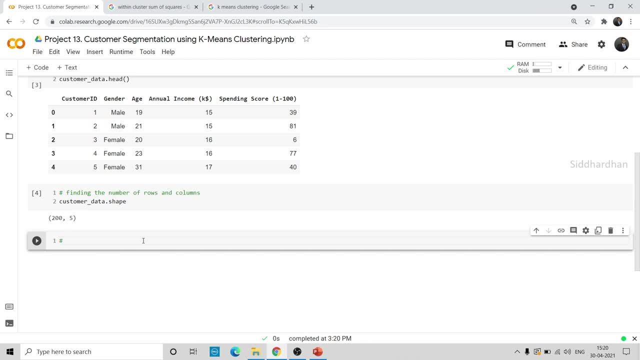 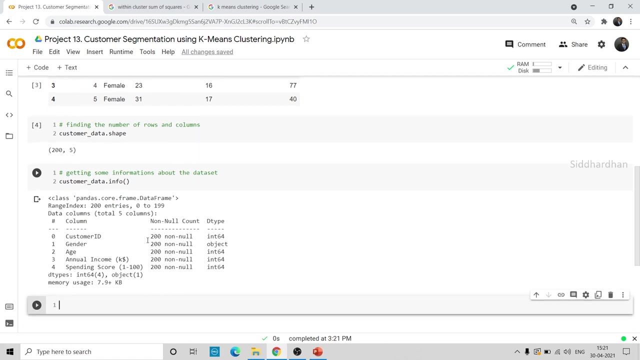 these are such kind of a drill which we used to do in a regular basis. so getting some information about the data set, okay, so i'll mention the data frame name: customer data dot info. so totally we have 200 entries. that means the 200 rows from 0 to 199 and totally 5 columns. so 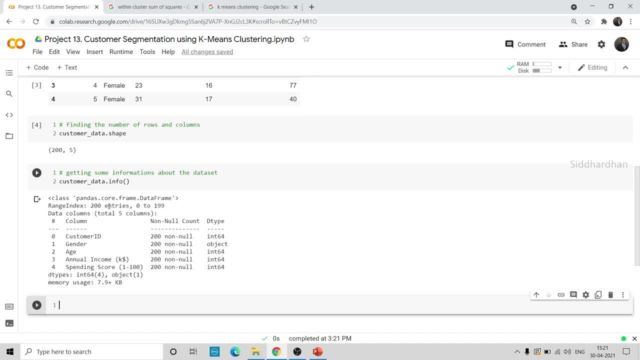 null value means, uh, missing values, and 200 non-null values means no values are missing. so that's what we are getting from this non-null value count, how many non-missing values we have. so that that's, uh, you know, given in this non-null count, and we also have the data type of each of the column, right. so? 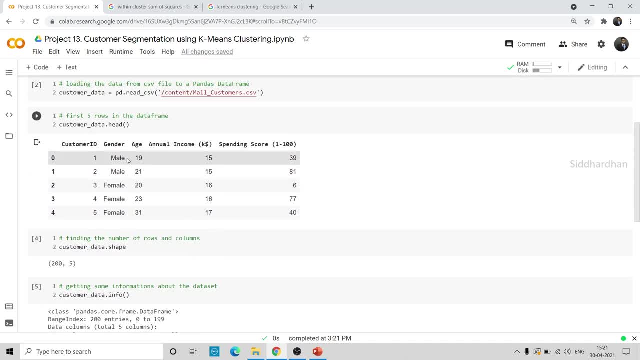 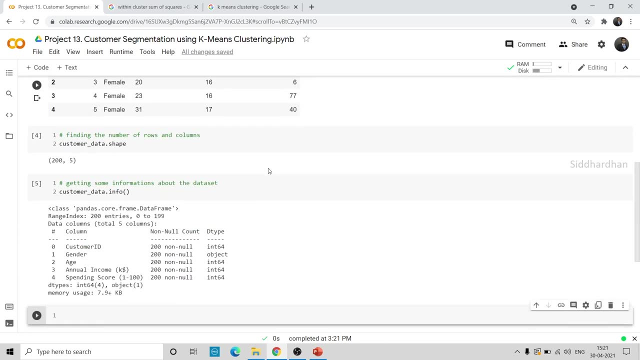 in 64 represents a 64-bit integer value. so, except this gender column, which have this string value, so this value is taken as object. so, other than that, everything is an integer data type. right, so this is how you can get the information about this data. so you can also get more information about. 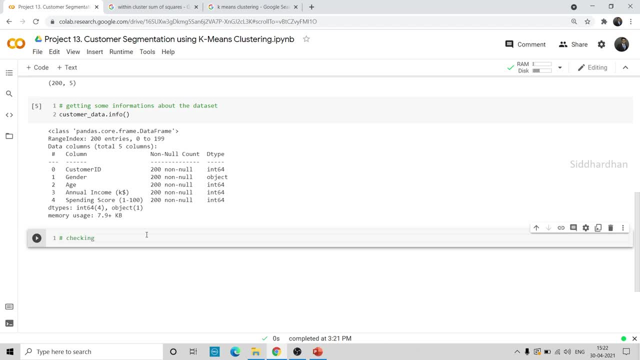 the missing values in a data set. so I'll mention a text here as checking for missing values. okay, so customer data dot is null dot sum, so this particular line of code will give the number of missing value in each column. so, as you can see here, we don't have any missing values in this case, which is a good thing. if we have any missing values, then 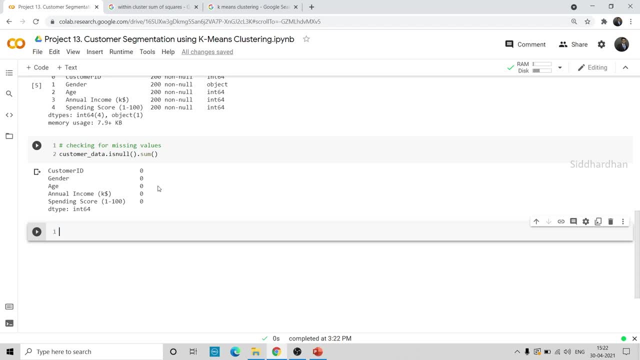 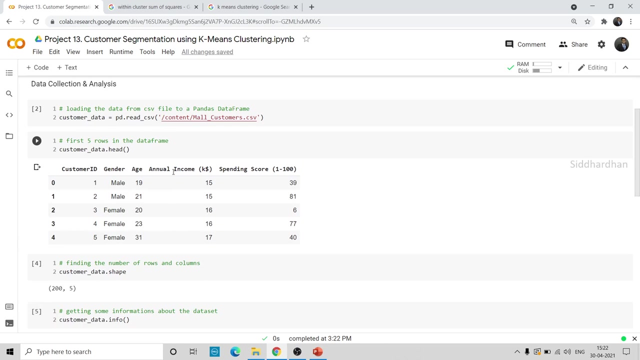 we follow methods like imputation to replace those missing missing values with suitable values. okay, so, as we don't have any missing values, we can proceed to the next step. right, so now we need to. we are going to choose which columns we are going to need, uh, you know, for our clustering. so, as you 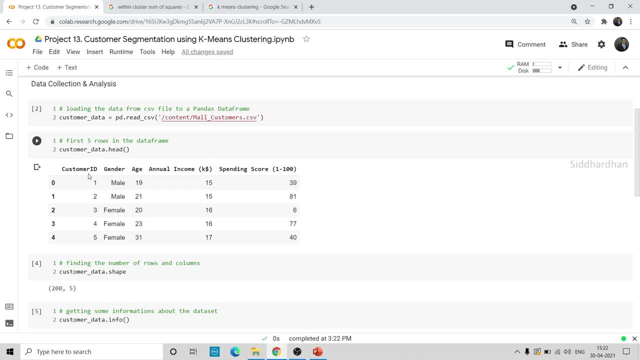 can see here totally. we have five columns. the first column is customer ID. so we don't want this customer ID. you know it's not required because we are going to group the customers based on their spending behavior and for that customer ID is not required. and also gender and age is also not that much required for this case. so you can also use. but 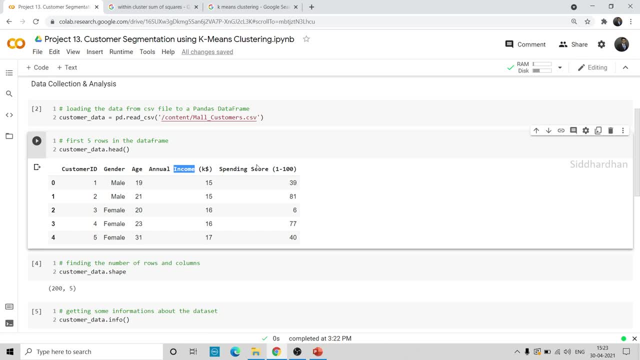 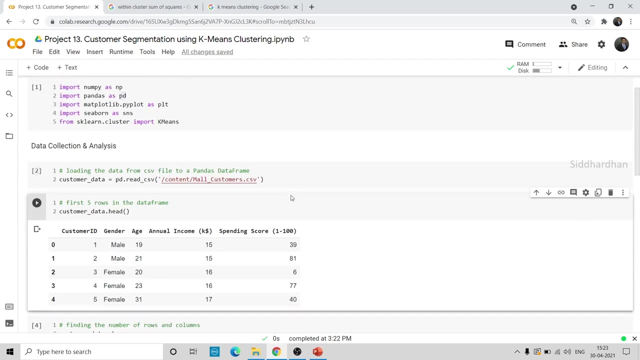 I'm in this case, I'm just going to use the two features: annual income and spending score. so what we will get is group of customers, and these groups of customers will be classified based on their annual income and spending score. okay, so I'm going to choose these two columns alone, okay? so now let's extract these two columns. 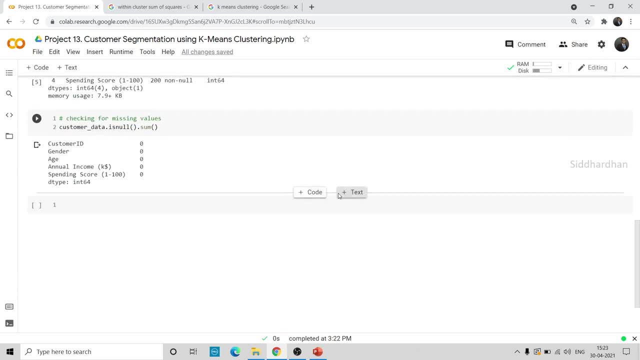 alone from this customer data. so I'll put a text here, choosing the annual income column and pending score column. okay, so I'll put a variable given a variable asset, so I'm going to take these two columns and store it in the variable X. okay so customer data and we need the last two columns, right? so for this I'm going to use the. 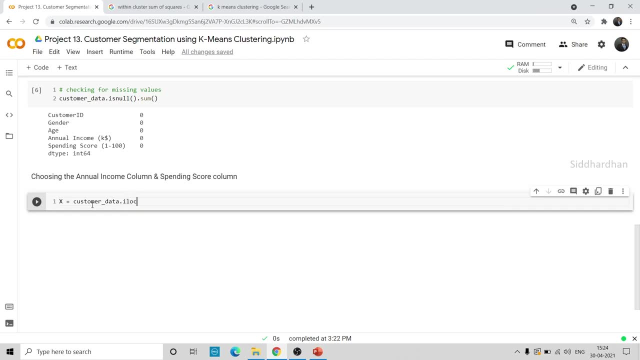 function. I look. so we are going to locate specific columns and for mentioning the columns we need to slice this data frame. so it's three comma, four dot values. so I'll explain you what we are doing in particular line of code. okay, so what we are doing is we are taking this customer data. so this is the. 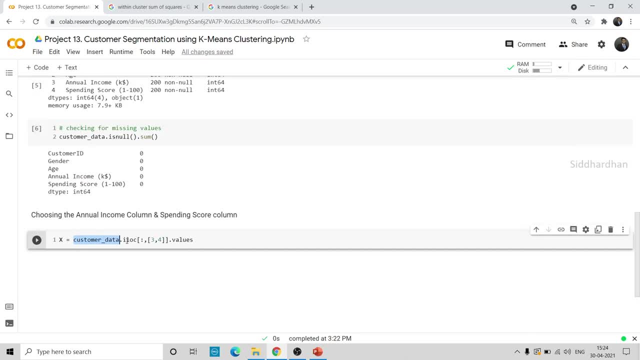 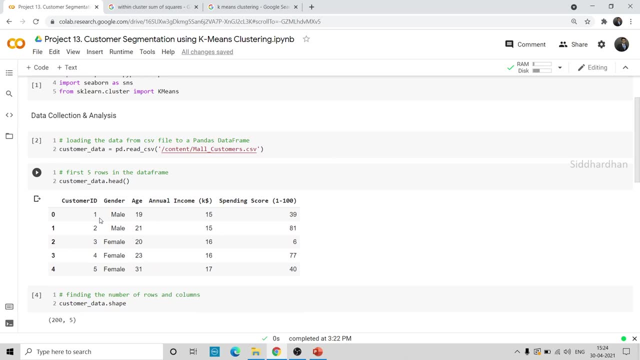 data frame- here we have right, so customer data, and in this we are locating particular columns. the columns are nothing but three and four. here indexing in python starts from zero, so it you know, number count doesn't start from one, but it starts from zero in python. so the index of this 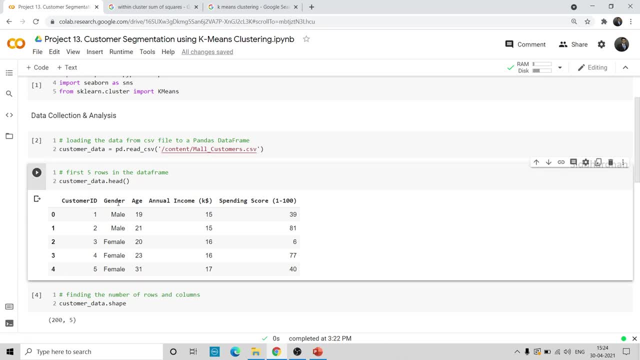 first column, this customer ID column, is zero and the index of gender column is one and for ages two, for annual income three and four. so totally we have five columns and this is zero: one, two, three and four. so we are going to take these two columns. 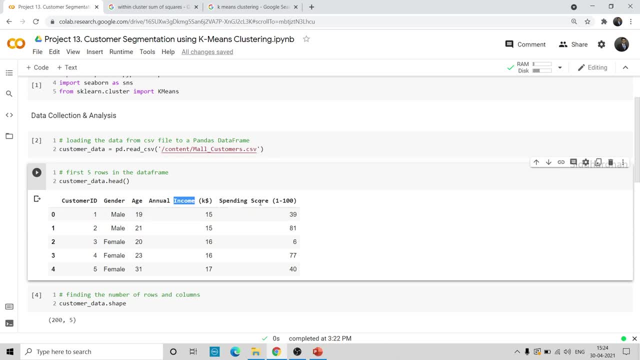 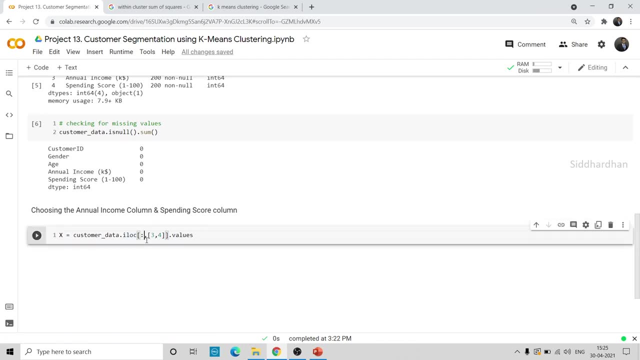 right. so the index of this annual income column is three and the index of spending score column is four. so i have mentioned this three comma four. so you can see here i have mentioned a column here and a comma here. that means i am taking a third and fourth column. that means you know the index. 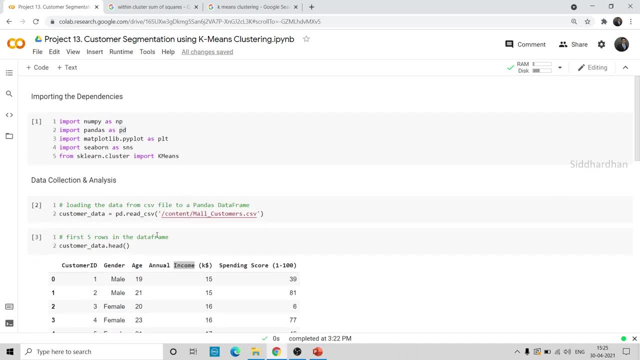 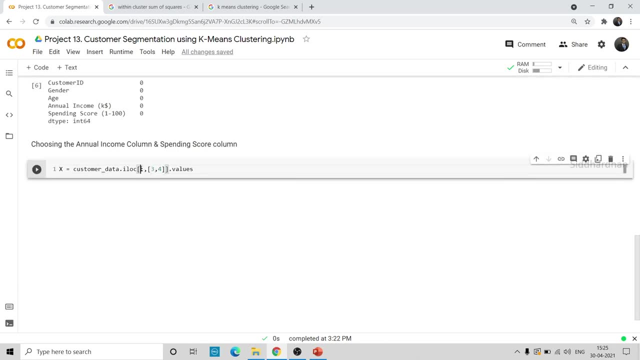 third and fourth column. if i don't mention this column column, it means that we are taking third and fourth row. so that is this particular slicing thing which we are doing here. so we are mentioning that i own this column with index 3 and 4, which are nothing but annual income and spending score. 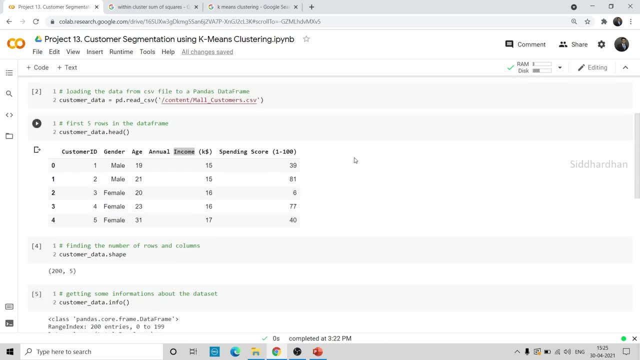 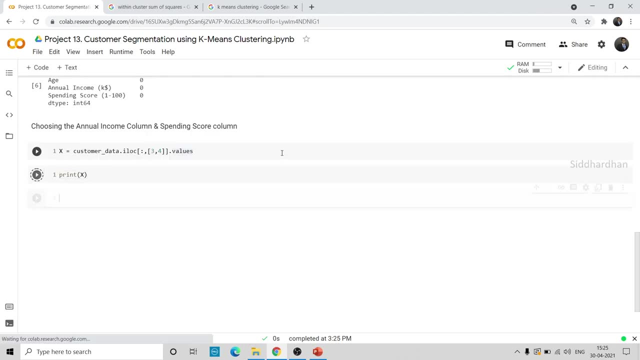 okay, so dot value. so i'm just going to take all the values, nothing other than that. okay, so let's run this. now you can print your x and see what are the values you have. okay, so, totally, we have a list of values and each list contains two values. the first value represents: 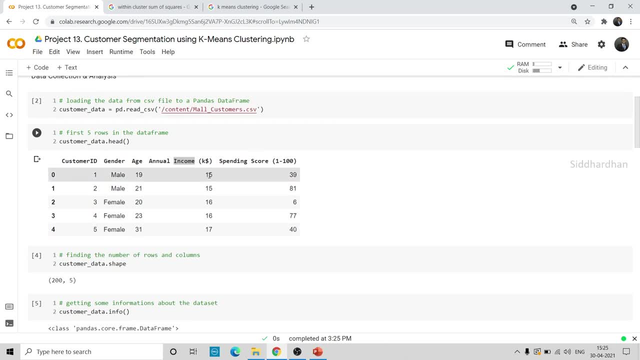 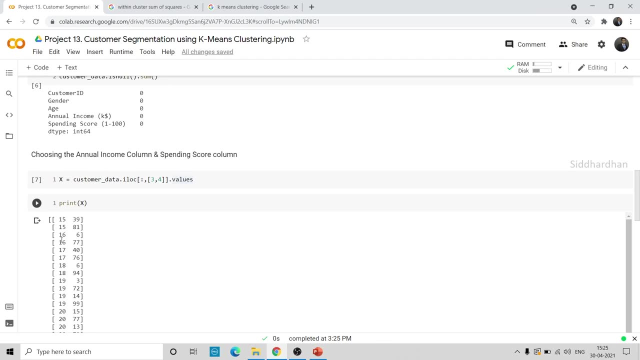 the annual income. so you can see here the first value here is annual income, 15 and spending score is 39. you can see here: 15 and 39. so all the values in this first column represents the annual income of specific customers and the second value in each list represents their spending score. so these two 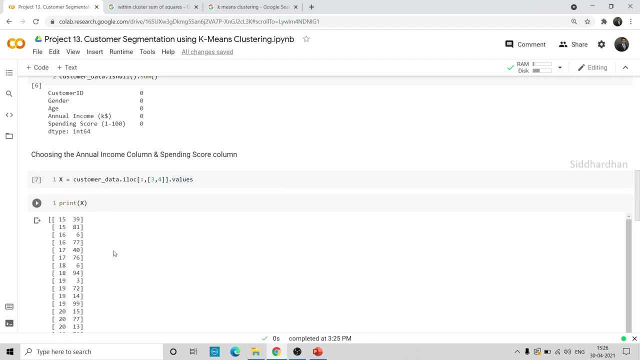 values are the ones which we need for our clustering. okay, so in our x axis we will- uh, you know- take their annual income, and in y-axis we will take their expanding score. so that's why we need these two ones, in the sum of the values of each, and then we will go ahead and do another. 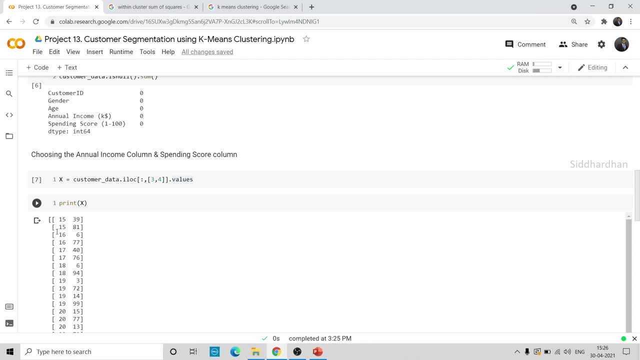 values alone, so we won't be taking any other values like their age or gender. so we will just take these two values, okay, so now what we need to do is so, as I have mentioned before, the next step is to choose the correct number of clusters. so, choosing the number of clusters. 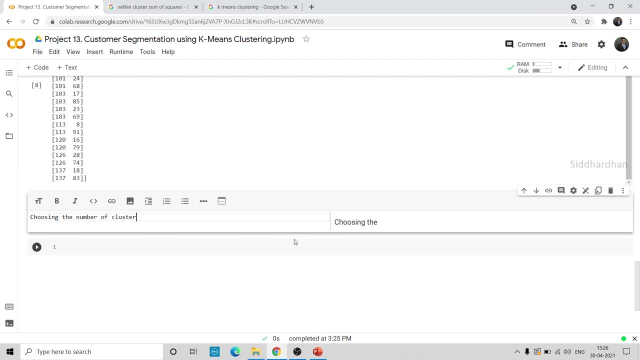 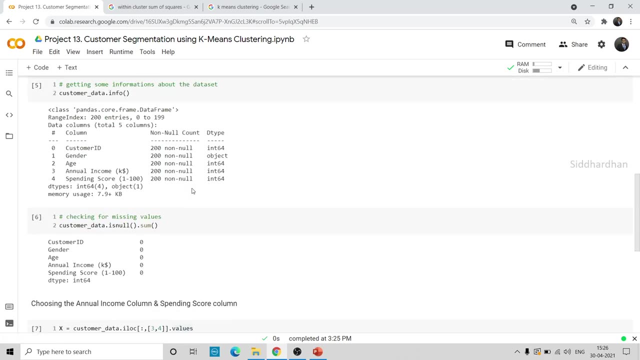 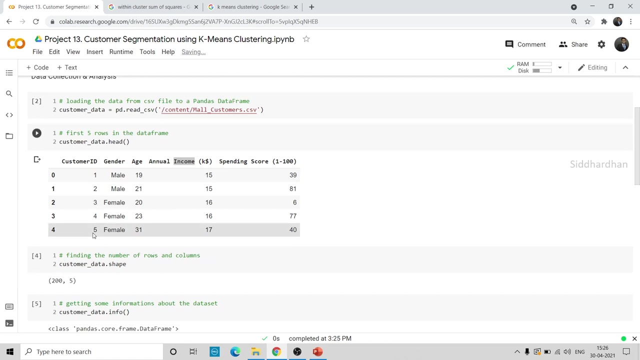 so in this case, we don't know that whether we need to choose. I'll just remove this for now. okay, so we don't know for this particular dataset. so totally, we have 200 data points or 200 rows. we don't know that how many clusters we can make from this data, right? 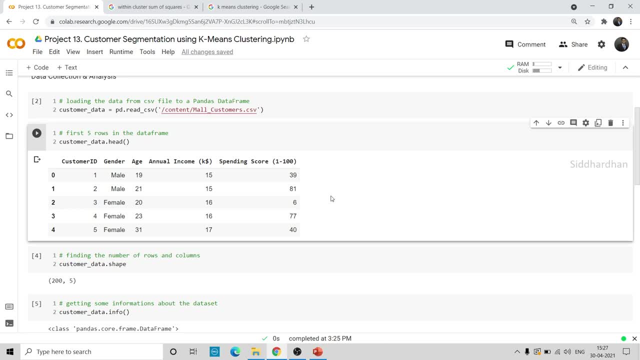 so we can make three clusters or four clusters or five clusters, any number of clusters, but we need to find what is the correct or what is the optimum number of clusters, that is stroke for each of them. So we don't know how many clusters we can make from this data. Okay, 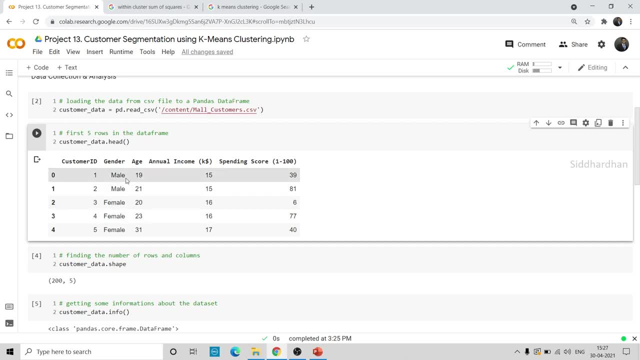 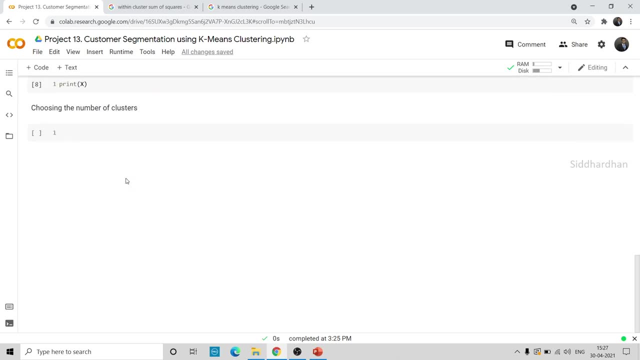 suitable for this data set. so this number of clusters varies depending on the data set. if you are dealing with a different data set, then you need to, you know, choose a different number of clusters. so we will choose the correct number of clusters by using a parameter and this parameter. 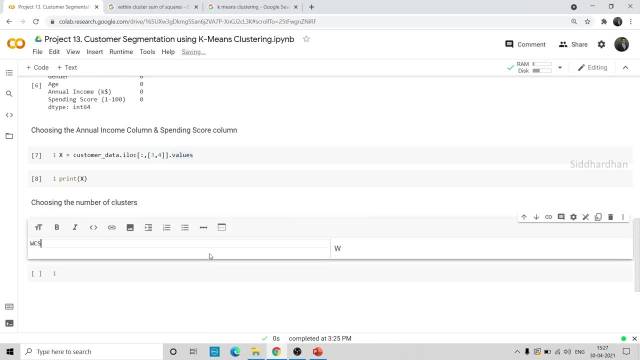 is called as wcss and wcss represents within clusters, sum of sqaures. okay, so you can search in google if you want to get more information about this: within clusters, sum of sqaures. i'll just explain you what is meant by this so you can see here. 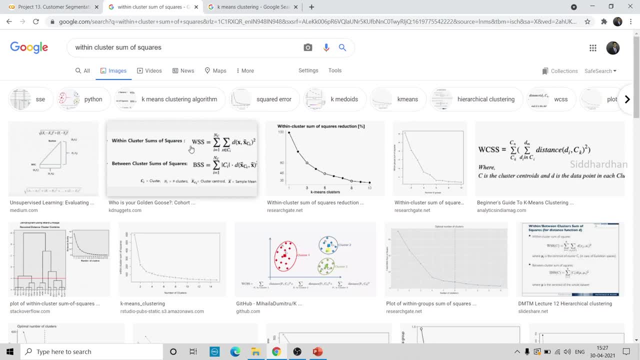 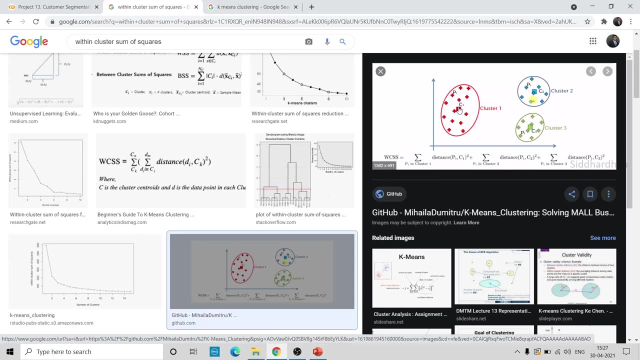 this is the formula for finding this within cluster sum of sqaure value. so it, you know, tends to find the distance between each data point and their centroid. so you can see here: so the plus symbol represents each data point. so here we have x right x, else minus xeta. so this is the plus symbol here and here it's written on thene of the data. 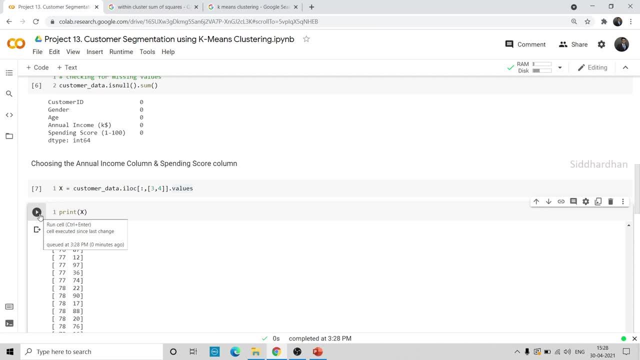 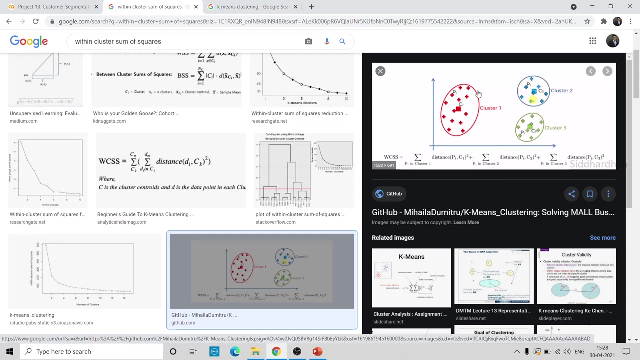 here the x represents. so i will just run this here: x represents. so the first value, or the x axis value, represents the annual income and the y axis value represents their spending score. similarly, if we take our annual income in x axis and y axis, we will plot all the data points in 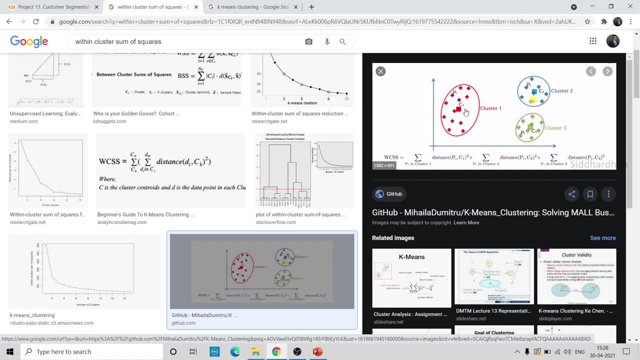 this graph and plus represents all these data points, and this, this square, represents the centroid. so each clusters have as their own centroid. so in this case the number of clusters we have is three right. so when you try to find this wcss value, it tries to find the distance. 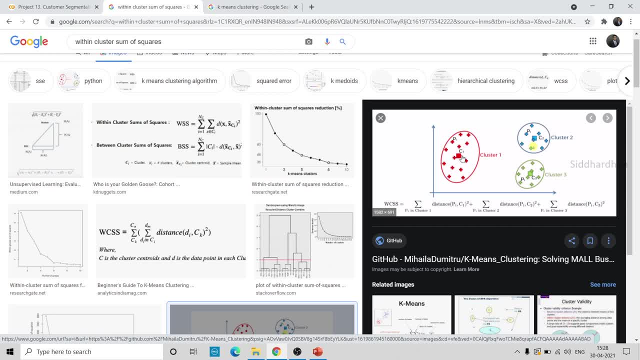 between each data point and the centroid of those clusters. okay, so for a good cluster, this data points should be, you know, very close to this particular centroid. so that means the we get good partitioned clusters. okay, so, as you can see here, in this case these data points are close to. 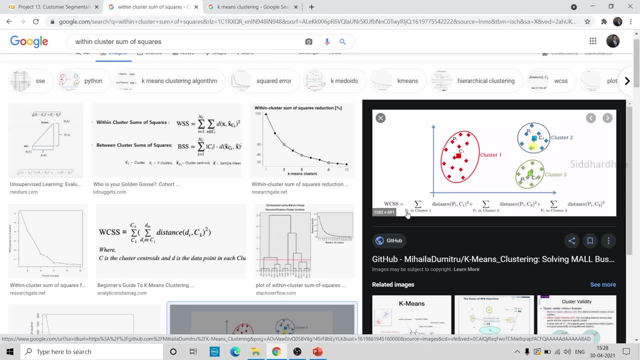 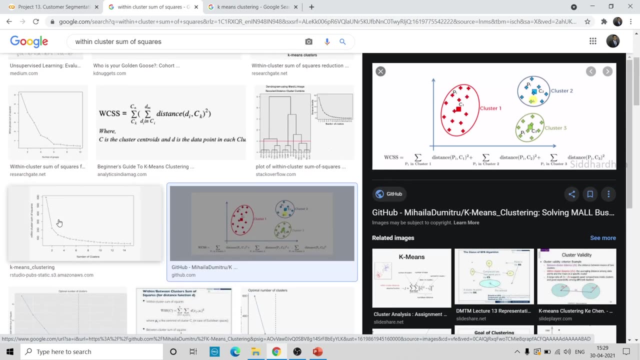 this cluster and it is the similar in this case as well. so when you have the correct number of clusters, the wcss value should be very less. that means the distance between the data point and the centroid should be very less. for this we will find this wcss value and, you know, build a plot like this so you can see here this plot or this. 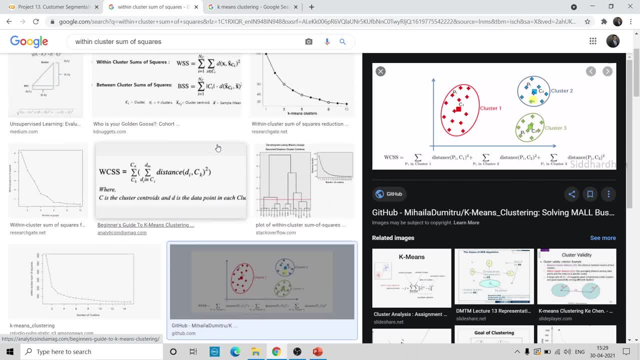 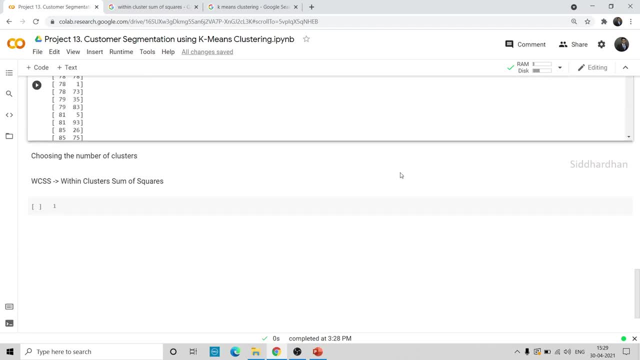 graph is called as an elbow graph. so in this elbow graph we will see which number of clusters has minimum wcss value. i'll show you how we can find this. so this is called as elbow method, so i'll just make this a little bit more simple. so i'll just make this a little bit more simple. 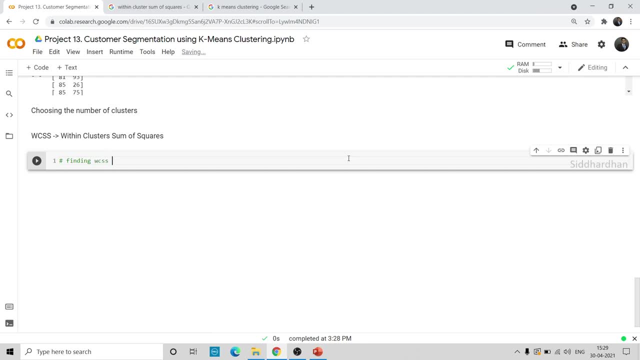 this is finding wcss value for different number of clusters. so in this case we are going to create a for loop and in each cases- so in the first case we will find the wcss value when we consider for only one cluster- then we do it for two clusters, then three clusters, all the way up to 10 clusters. 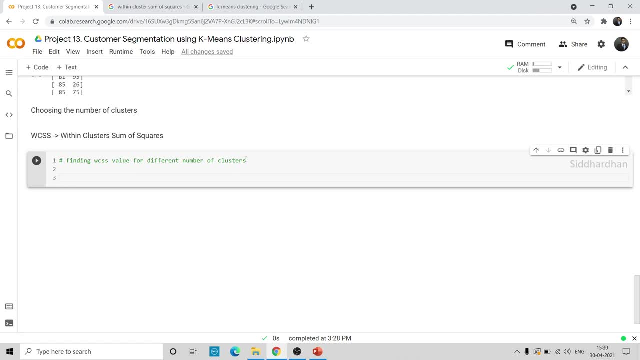 and in this 10 clusters, we will try to find for which number of clusters there is minimum wcss value. so this is the end result that we want for this particular step. okay, so i'll create an empty list as wcss. so i'll create this empty list. now we can create a for loop for i in range. 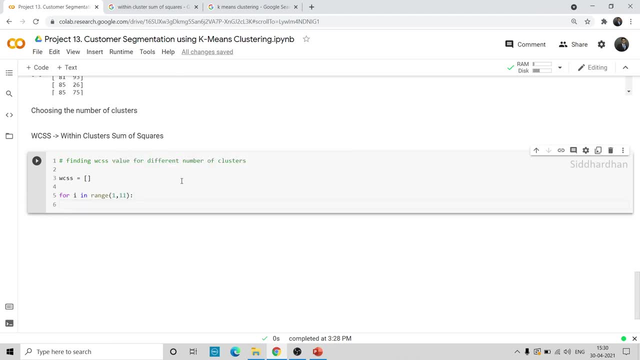 1 comma 11. okay, so 1 comma 11 represents i will be taking values from 1 to 10. so when you mention, you know, two numbers inside this range, key word, it takes this first value. so here the first value is 1 and the second value is 11. 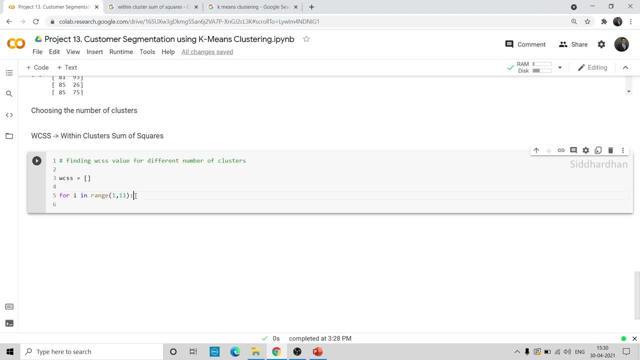 so it is like n minus 1, so it will take all the values from 1, 2, 3, 4 and up to 10, so this second number won't be included. so if i mention, you know, 1 comma 20, then it takes. 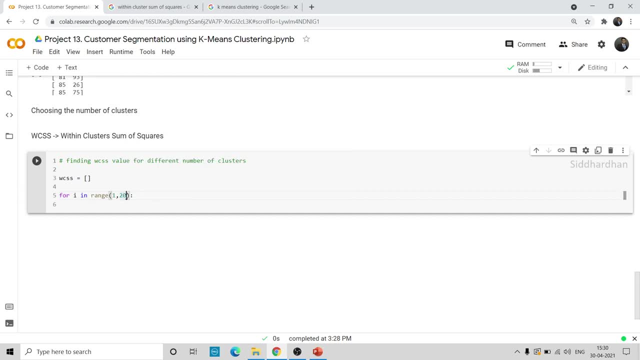 the number of clusters from 1 to 19, so the second number will be excluded. so here i want the number of clusters to be 10, so it will be checked for one clusters, two clusters, all the way up to 10 clusters. so i need to mention 11, because this 11 will be excluded, right for that purpose. so for i in range: 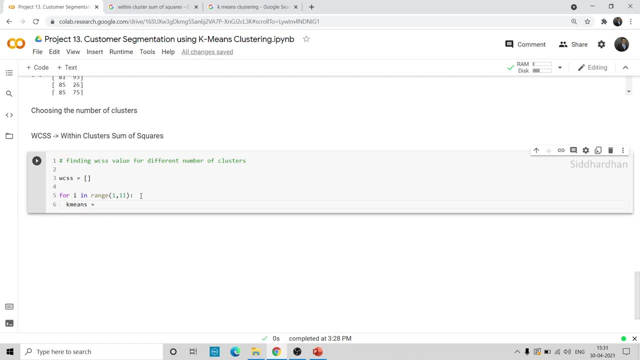 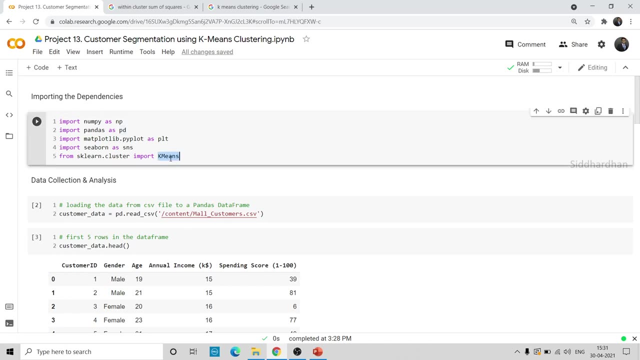 let's create a variable as k means and this k inside. this k means we are going to load the k means cluster function which we have. you know this is the k means clustering model. so i'm going to use this k means function and i'm going to load it inside this k means variable. 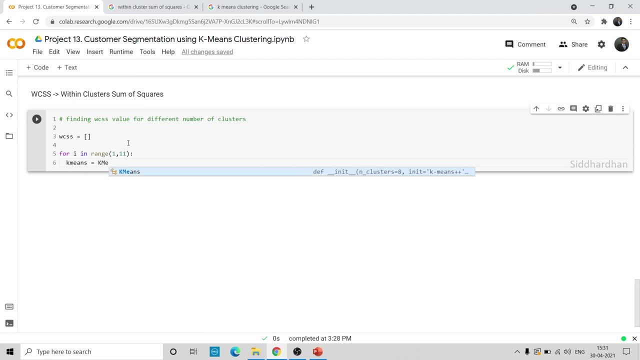 so k means is equal to. so k and m should be in caps k means. and inside this we need to mention the number of clusters we want. so you can see all the parameters. okay, so the first parameters is n clusters. so the number of clusters we want is i. so the first time this for loop runs we will take. 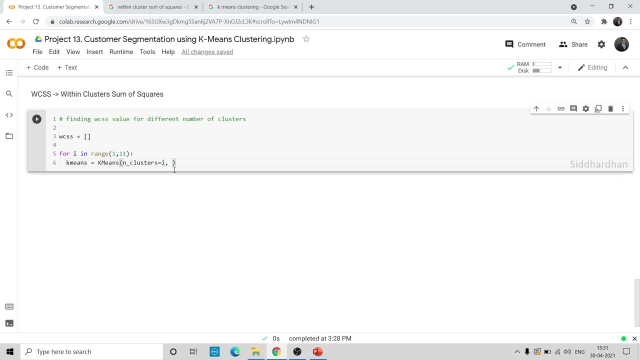 the value 1, so in this case the value become 1, and once this, once this for loop is completed, again this particular for loop will be carried out and in that case the value will be 2 and in that case the n clusters will be 2, and similarly the process goes on. so it is, you know, a simple. 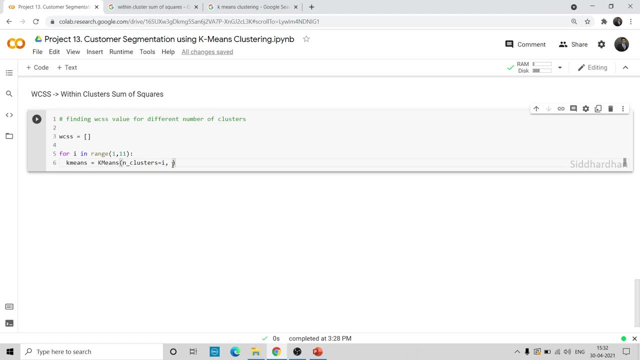 way of our for loop works. so n clusters is equal to i and the initiation step which we are going to use is k means so k means plus plus okay. so there are other initiation steps like froggy initiation and random partition initiation, and the best initiation method is k means plus plus. 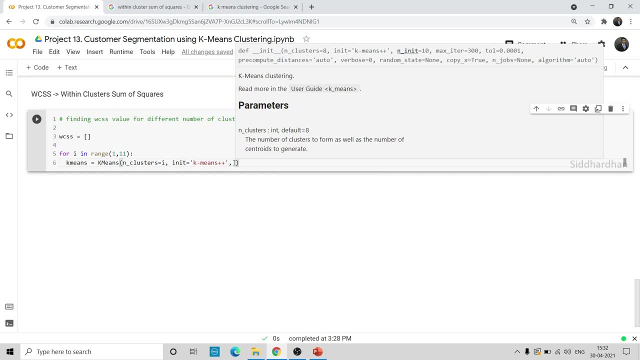 when it comes to k means clustering, so you don't need to worry about all these things in this video. so i'll you know. in future videos i'll be making uh videos on machine learning model, where i will be explaining you how a machine learning model works. like you know, a k means 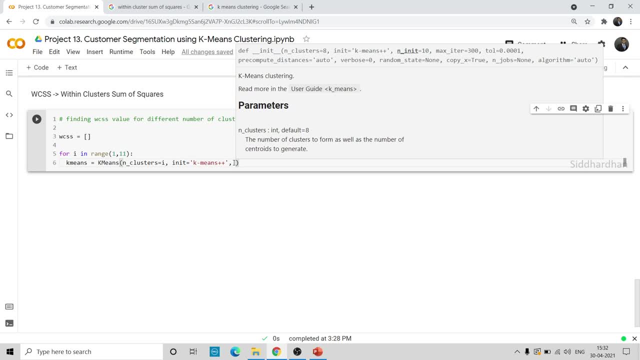 clustering model. so i will be explaining you how this model works and what is the math behind this model and how we can build these models from scratch, those kind of things. so in that i'll explain you in detail about uh, this model. the purpose of this video is to understand how we 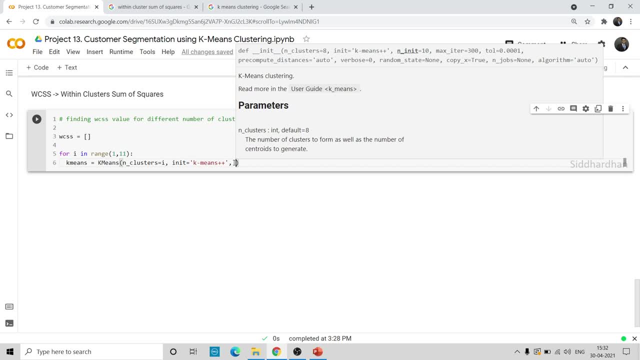 can implement this model in our projects. okay, so you don't need to worry much about this. so you can understand that the good initiation method is the one that we are going to be using in this video. so the method is: k means plus, plus, and for finding the number of clusters we can use this. 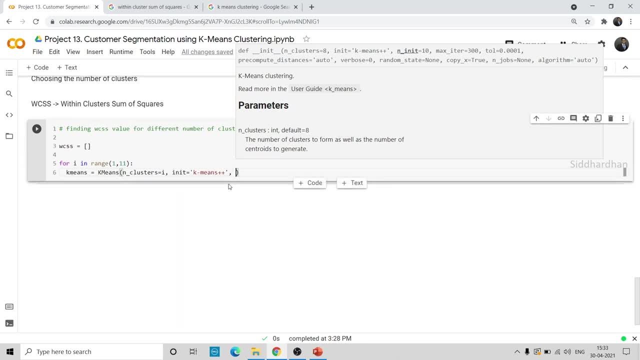 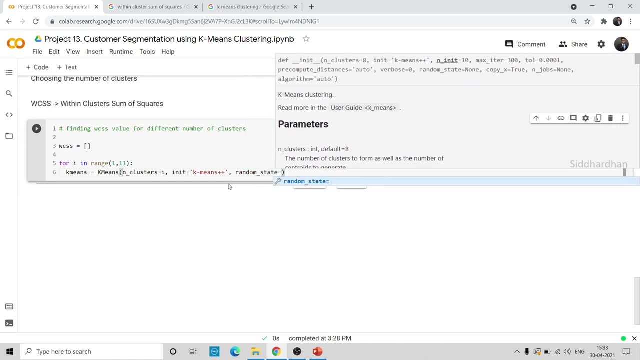 within cluster. sum of square value. okay, so the next parameter we need is random state. so random state is equal to you can give any number, so i'll just give a random number as 42. so, like this, data will be taken in a random fashion when you do this kind of processing. 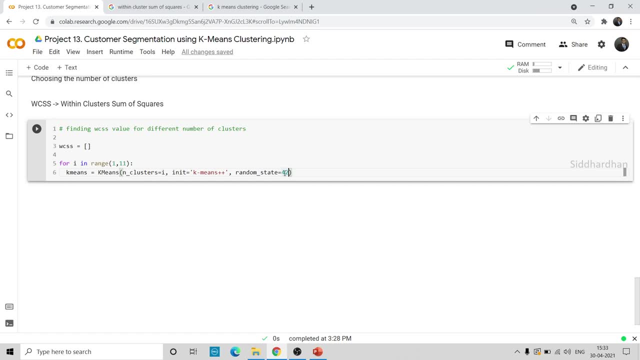 so here i mentioned this random state 42, right? so if you mention some values like one or two, then the way your data is arranged will be different. okay, so if you mention the same number as here i mentioned 42, if you mentioned the same number, 42, then your data will be splitted in the same way that my data is. 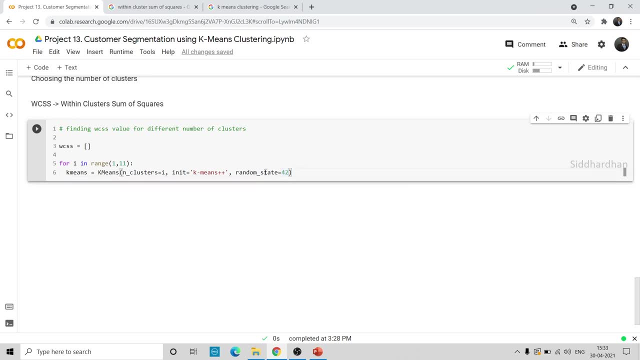 splitting. so this is just for the reproducibility of code, so this is not that significant in this case. okay, so the significant things are this number of clusters and the initiation method which we are using, and then we need to fit this k means to our data. here our data is: 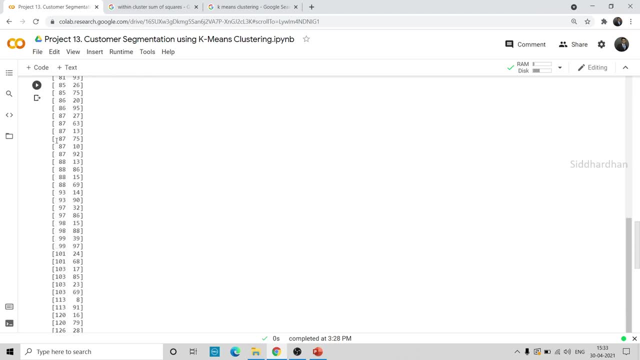 x, right, so here x represents the annual income and this uh pending score, right. so we have loaded that data index, so we need to fit this data to this. k means so, k means dot, fit x, and now we need to find: so. this will give us the wcs value. 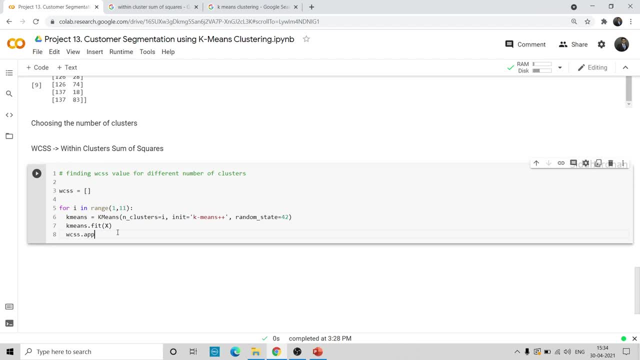 so wcss dot append- i'll just make a space in- so wcs dot append. k means dot inertia, k means dot inertia. okay, so this k means dot inertia will give us the wcss value. so this particular in area inertia function lies in this. k means algorithm, so when you do this it will give us the wcss. 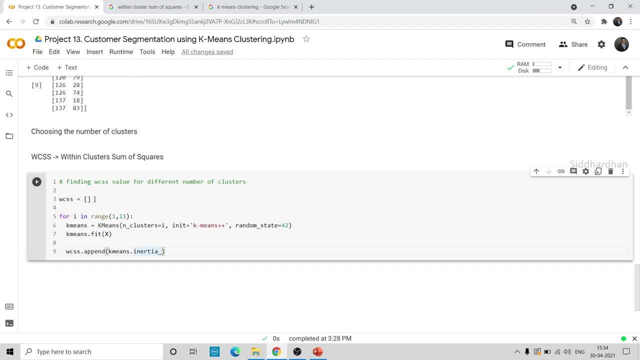 value for each clusters and this value will be stored in this list. so in the first case, when this for loop is running this, i will take the first value, which is one, and this i goes here. so i'm splitting the data as only one cluster, it's only one group, and it will feel this. 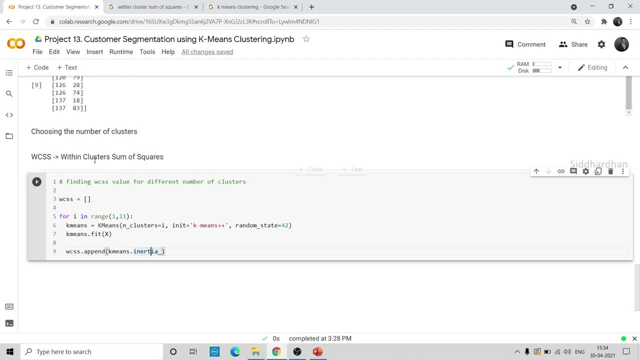 data and it will find the wcss, the within cluster sum of square value, and it will put that value in this particular list and once this for loop is completed, then it will again, you know, carry out this loop again. now it will take the second value, which is two. now the n clusters value will be two. 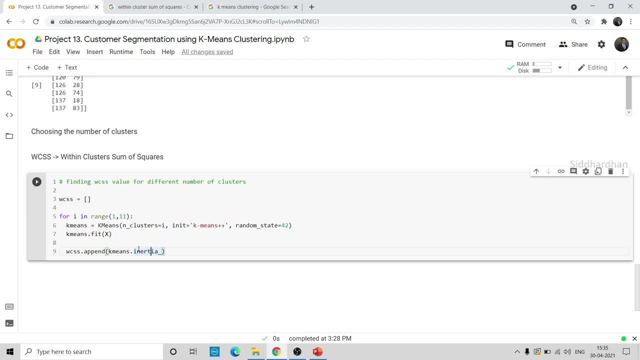 and again this will be created and now it will run and it will give the wcss value for two clusters and this process will be carried out until we do the same up to 10 clusters. okay, so i'll run this now, as i have told you before that we will create a similar elbow graph to see for which number of 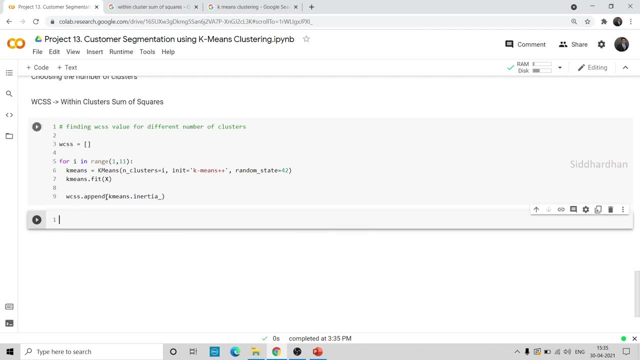 clusters we get minimum uh sum of square values. okay, so now i'm going to create a elbow graph. so plot an elbow graph to find which cluster has minimum value. so we have already imported the seaborn library, so i am mentioning same. so we have imported seaborn in the short form as sns. 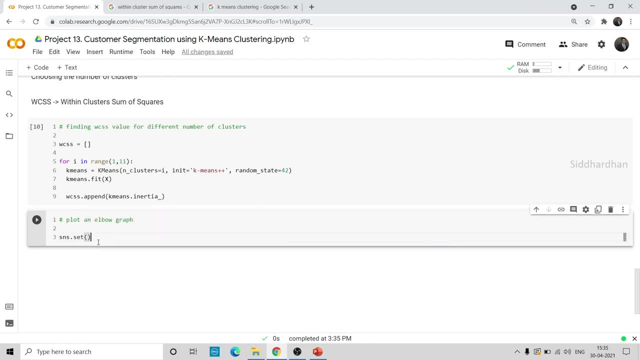 snsc it. so this will give the basic themes and basic parameters required for the graph and then i'll create the plot as plt dot figure. okay, so plt dot here, and okay, so we don't need to mention this. so plt dot, plot dot, range. range is the same, which is 1 comma 11, so this value will be taken as x-axis. so value from 1 to 10: 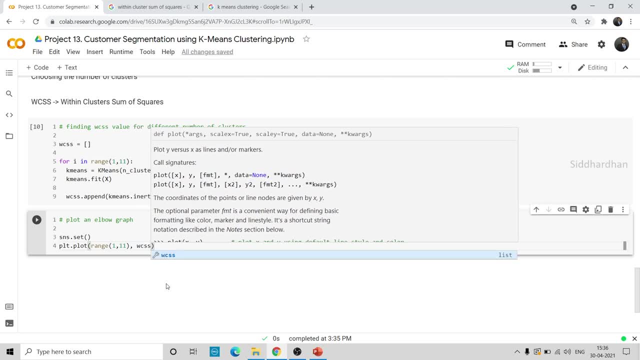 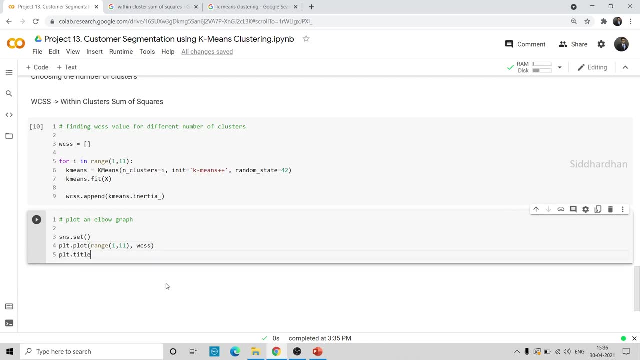 and the y-axis value is the list which we have within cluster sum of squares. now you can give a title to your plot: plt, dot title and the title is nothing but the elbow point graph. okay, and we can give the x label as plt dot, x label. 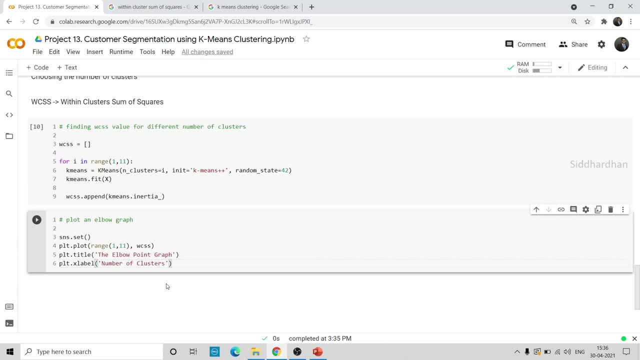 number of clusters. okay, so the y-axis label is plty label. one second, i'll just check this. okay, so the y-axis label is w css and finally we can show our thought plt dot show. okay, so let's run this. this will give us an elbow graph. so this is the elbow point graph, or you can. 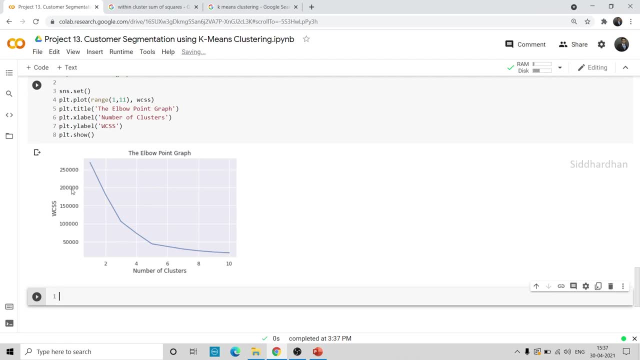 also call this cutoff point graph. So in the y axis we have this within cluster, some of spire values, and I have told you that this value should be minimum for the optimum number of clusters. and in the x axis we have the number of clusters, So 1, 2 in the middle. 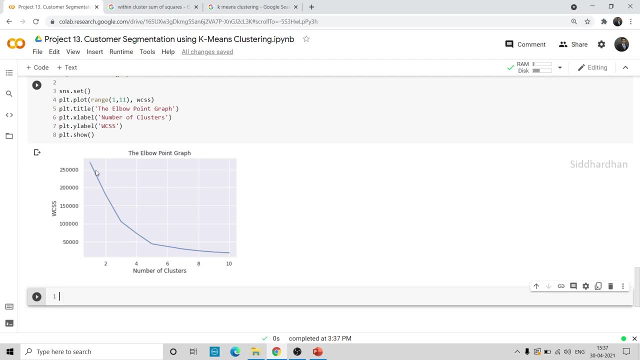 we have 3,, 4,, 5,, 6 and all the way up to 10, right? So when you analyze this graph, so there is a cutoff point here, So there is a certain drop in the value here for this. 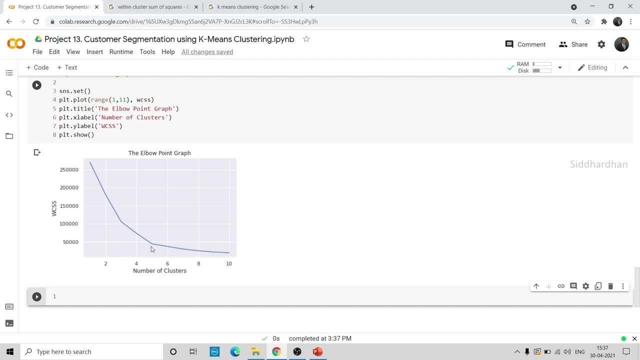 number of clusters is 3, and there is also another drop in the value for the number of clusters 5.. So now we have 2 ELBO points, So these points are called as ELBO points, and in this 2 ELBO points we will take this particular value. So here the value is number. 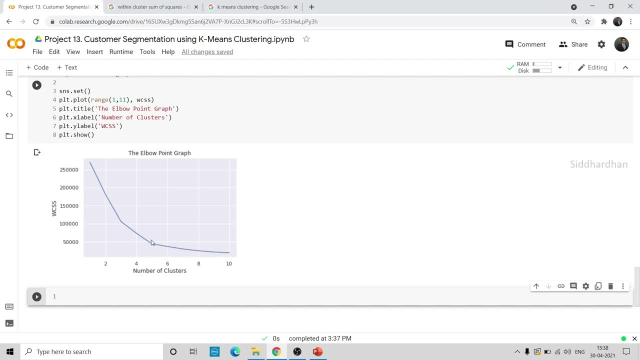 of clusters is 5, because after this there is no significant drop. right, So there is no sharp significant drop. So the correct optimum number of clusters we can choose is 5.. So this is how you can interpret an ELBO point graph where we will see, you know, the 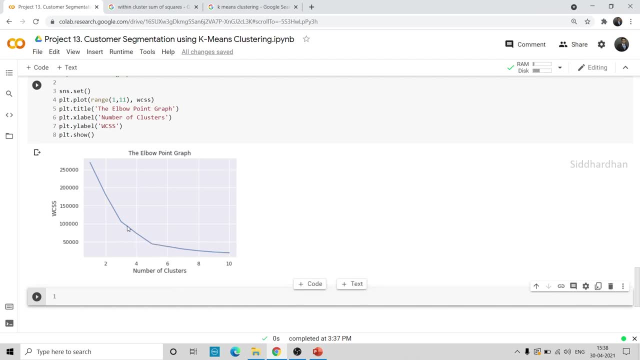 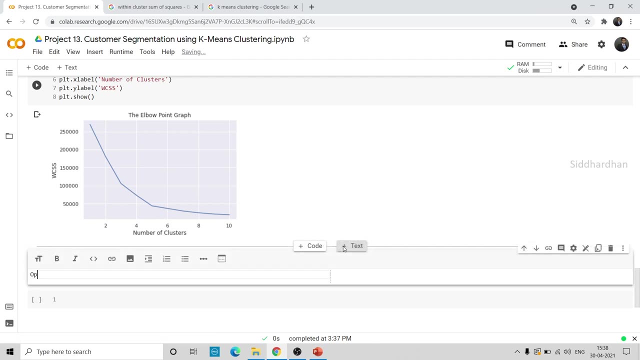 ELBO point, after which there is no significant drop in the value. ok, So now I am going to- I will just make a text here- as the optimum number of clusters- optimum number of clusters will be 5.. So we have interpreted it from our ELBO point graph. 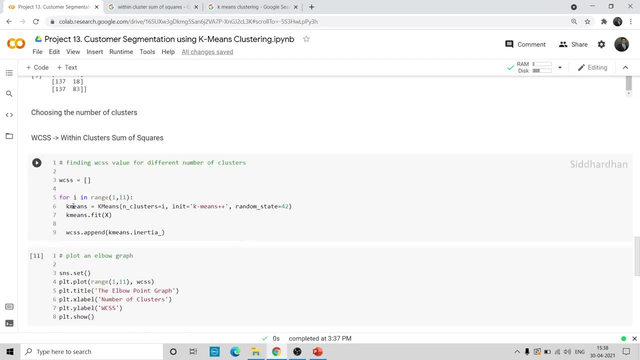 Now we just need to do the same thing. So we have already fitted this to the claimants clustering algorithm. So we will just do the same thing, but in this case we will give a say value to the cluster. So we have completed this Nou silly K file already, which we can. 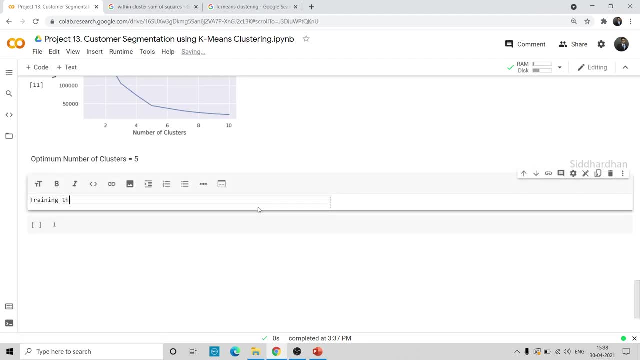 use for inongs and so on. So we just solve the sequence in our 한번RY Effect. Now let us comb it, for example. So come here, Let usuetc at where is now the new instructions for students to use the uncondeluble jullie straight rubber? الよろしく to normal. 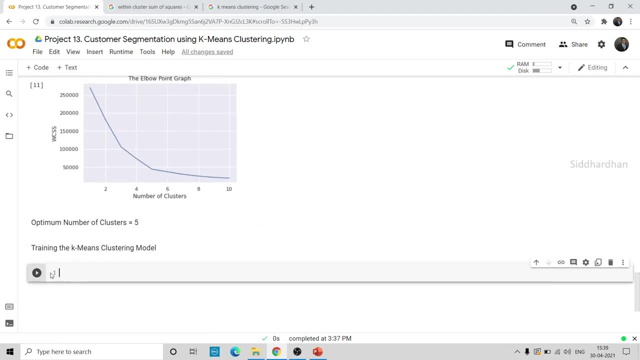 forgive, is equal to 5. ok, So this part is about training the K meanclustering model. So this is an example of an unsupervised learning model. K means clustering model. here K is nothing but the number of clusters we are taking. So k represents the number of 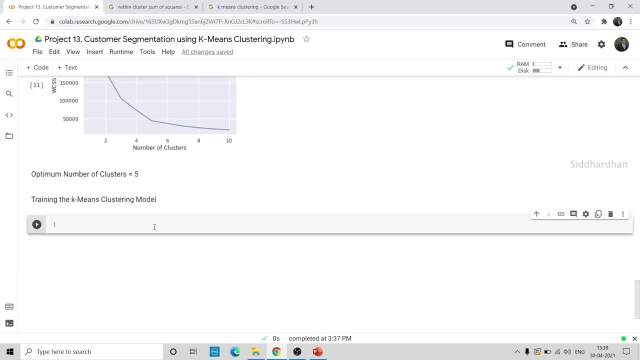 clusters and in this case, k. the value of k is equal to 5. ok, So welcome back. We will solve a creek script example of these problems in the coming. I will mention this. k means the same variables we took, so we have imported this. k means from: 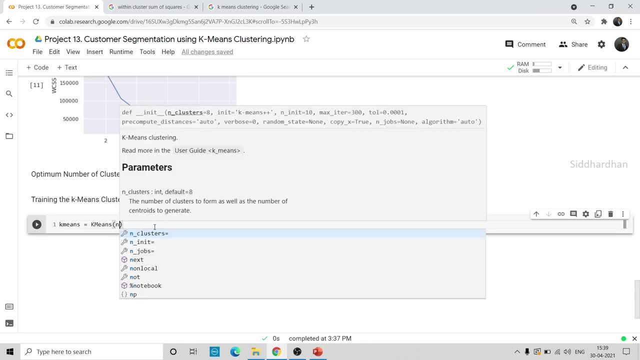 sklearnclusters, and inside this we need to mention n clusters, which is equal to 5, because we know the optimum number of clusters for this particular data set is 5 and initiation is k means plus, plus and again the random state, so you can mention any number we want. 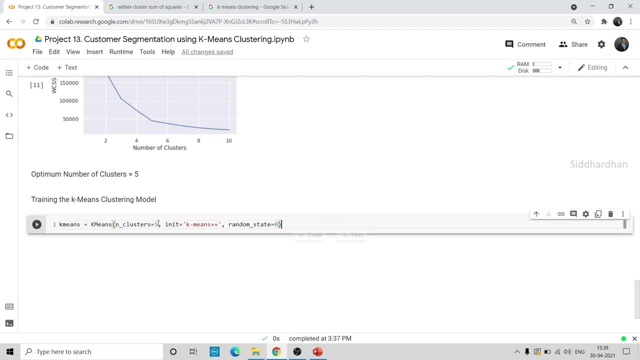 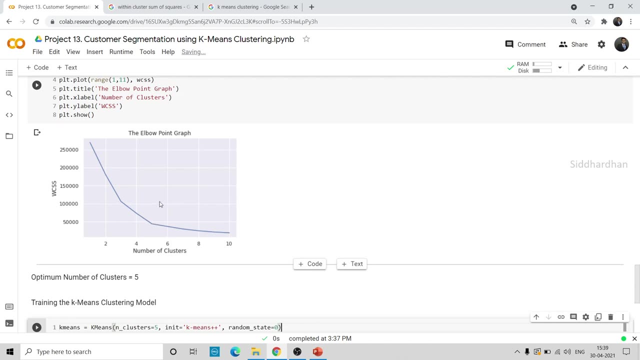 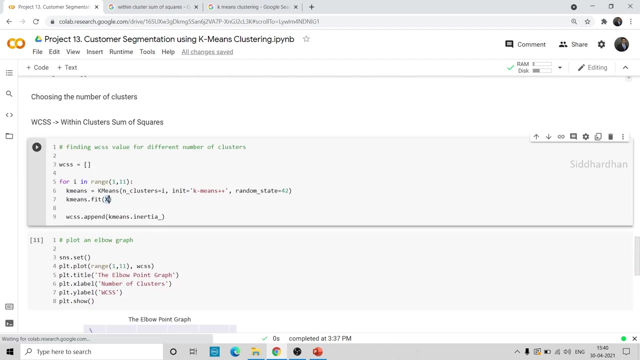 I will just mention it as 0. ok, So here we are taking 5 clusters. so this number of clusters varies depending on the data set we have. for this particular data set, the number of clusters is 5, so this is found by fitting the- this k means value- with x, right, so you can see, here we have fitted it with x. 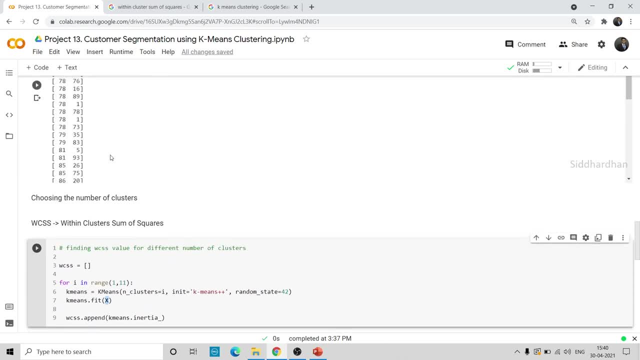 So this is the k means value and this is the k means value and this is the k means value. So this is the k means value and this is the k means value. So this particular graph depends on the values present in this particular x. so x is: 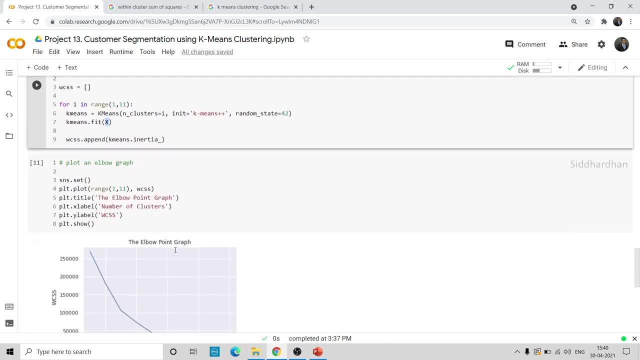 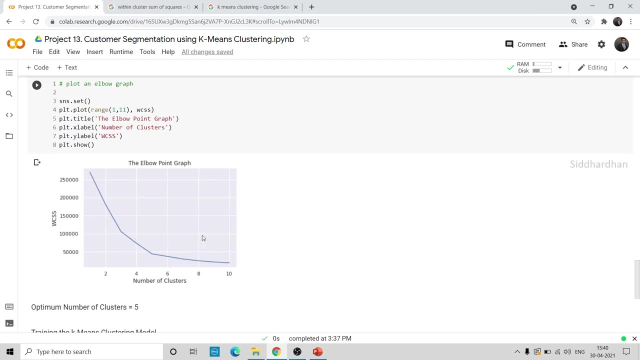 nothing but the annual income and spending score. right, if we have another data set. based on that data, we may get the optimum number of clusters as either 3, or it can also be 4,, 5,, 6 or any number of clusters, depending on the data set. so it is not the same, it is. 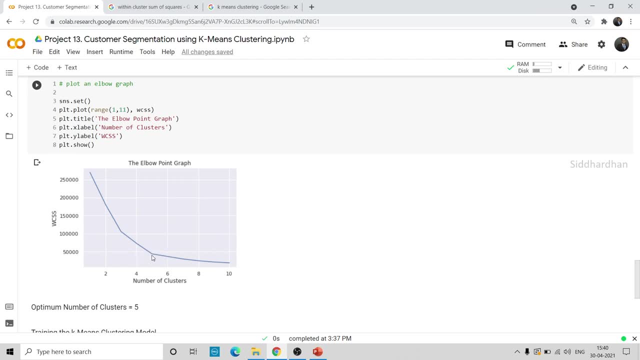 not that in each cases, in or in every cases, we will get the optimum number as 5, so it varies depending on the data set and for this particular data set it is 5. ok, so I have mentioned the minimum number of clusters is equal to 5 and this will load our k means model to. 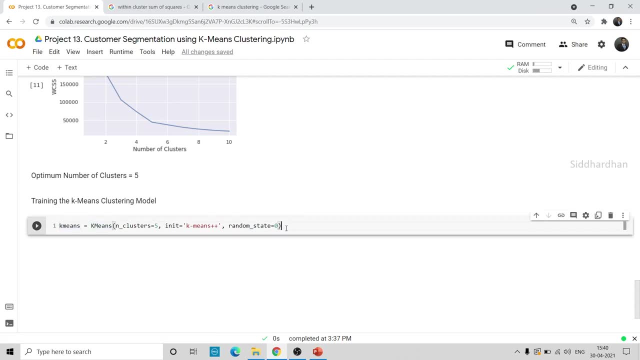 this variable, named as k, means ok. Now we need to return a label for each clusters. so I just mention it here: return a label for each data point, each data point based on their clusters. Ok, so what we are going to do is we will take all the values in this particular x, so 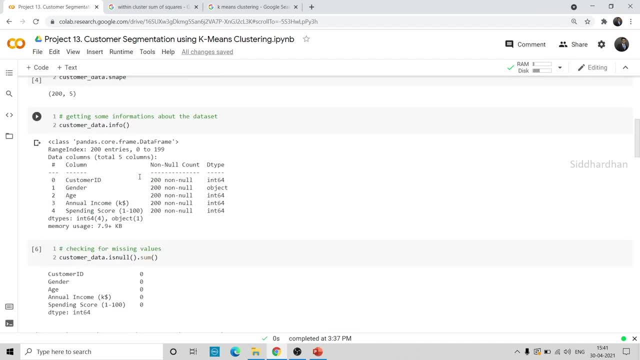 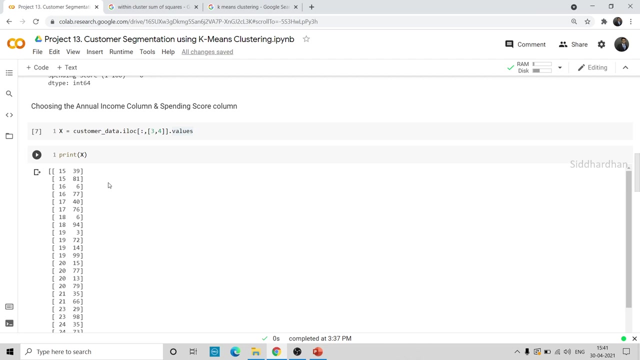 this x will contain 200 data points, because totally we have about 200 data points, right. so all these values will be splitted into 5 clusters based on their similarity values in annual income and spending scores. So each value will get a label. so we are taking 5 clusters, right? so each cluster will be given. 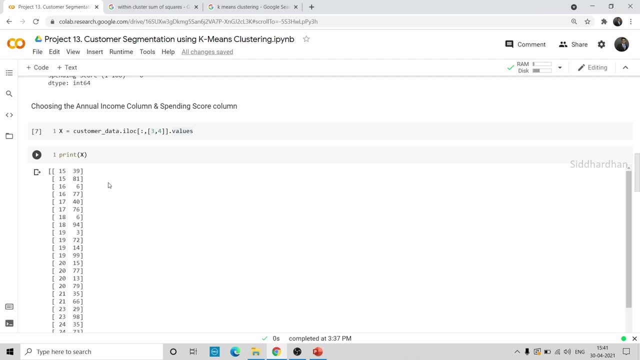 a label. so the first cluster will be given a label as 0. second cluster will be given a label as 0.. Similarly, we have 0, 1, 2, 3 and 4, so 5 clusters and each this data point. so this is one data. 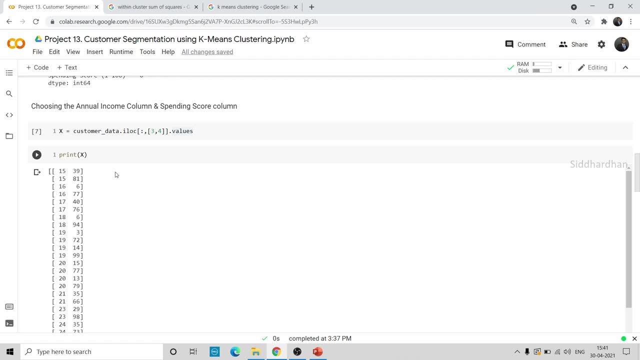 point and each data point contains two values, right, so they will get their own cluster number. so I will just show you here how we can get it. so we are going to return a label for each of the clusters, so let us store this label in a variable called as. y and k means is equal. 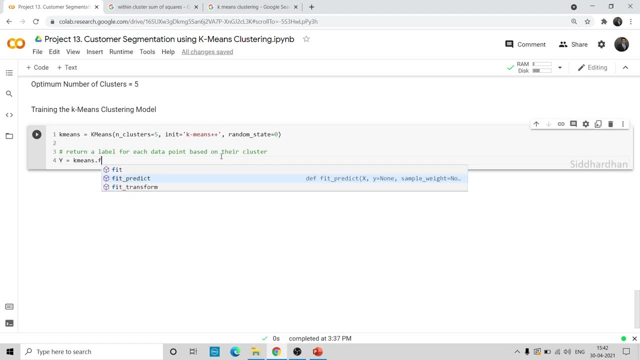 to k means dot, fit predict. So this fit predict will return a cluster number for each of this data point. ok, so fit predict x. so we are fitting all the values of x and finding which clusters they are belong to. ok, so now let me print this y. so let us run this. so as you can see, here we have several. 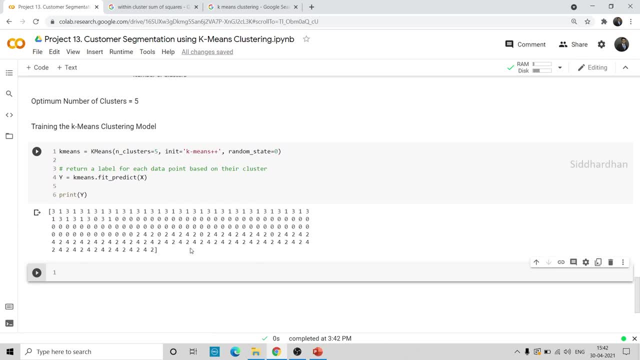 values, and the values are nothing but 0, 1, 2, 3 and 4.. So there will be 1, 2, 3 and 4.. So let us run this. So, as you can see, here we have several values, and the values are nothing but 0, 1, 2, 3 and. 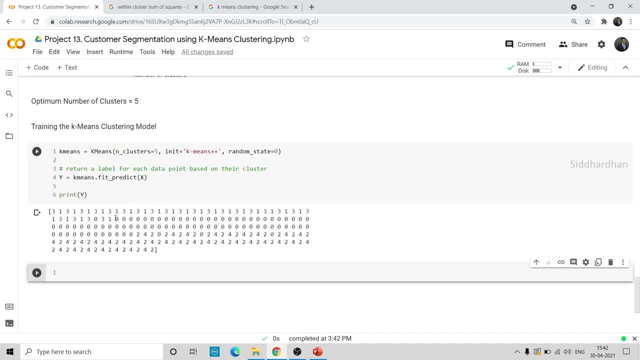 4. So we have only 5 values, because we have mentioned that we need 5 clusters. so all the data points with the cluster 0 are 1 cluster, and all the data points with the value 1 represents 1 cluster, and similarly 2, 3 and 4, so they represents 1: 1 cluster. ok, 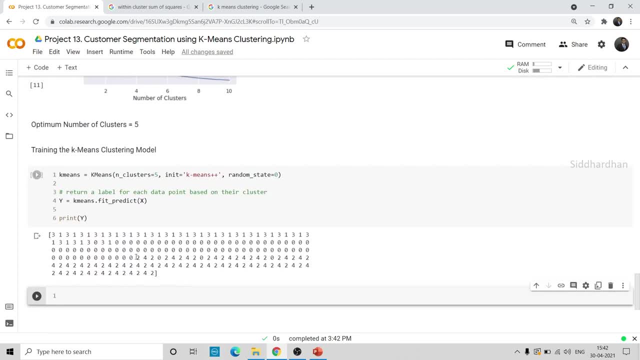 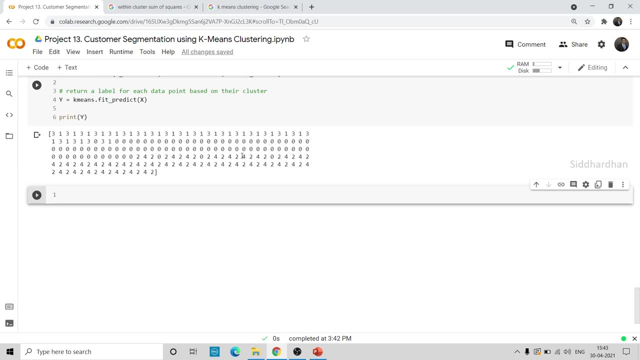 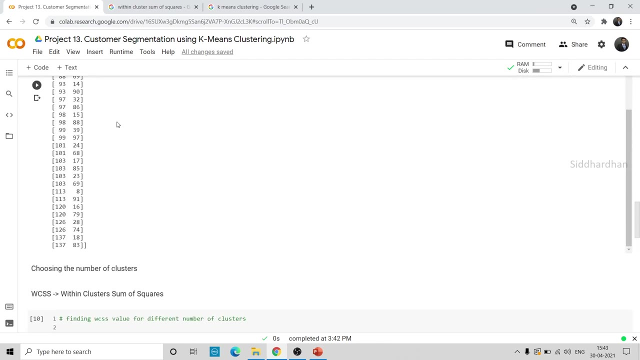 So this is the cluster number, so the cluster in which they belong to for all the x values. ok, so these are the clusters they belong to. Now what we can do is we can plot the data So, along with their cluster number And along with their annual income and their spending score, to see how this data is looking. 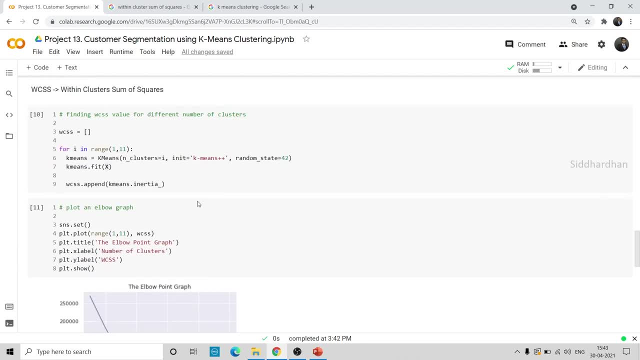 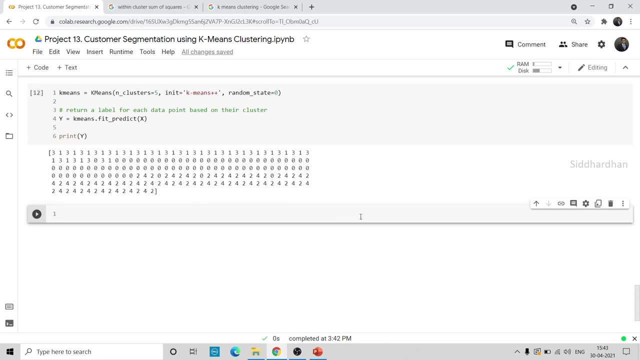 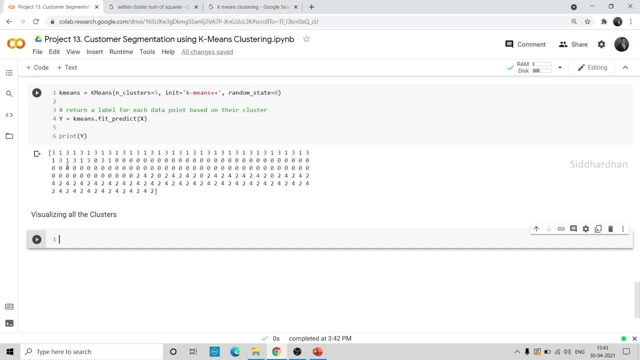 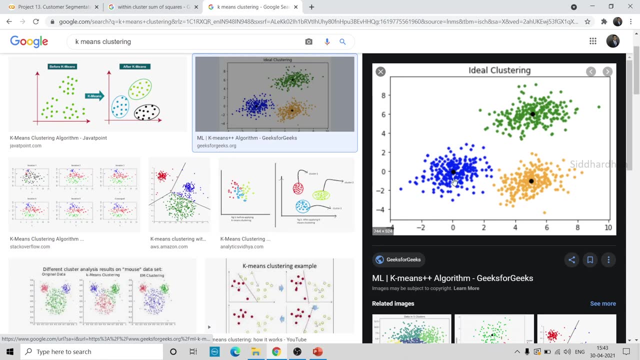 more into and we can get more intuition about this when I make a separate video about k means clustering. So you can see here, this is how k means clustering: clusters data. so these black dots are nothing but centroids. I have also mentioned you about centroid. So so, so totally. we have three clusters set and each cluster has their own centroid. 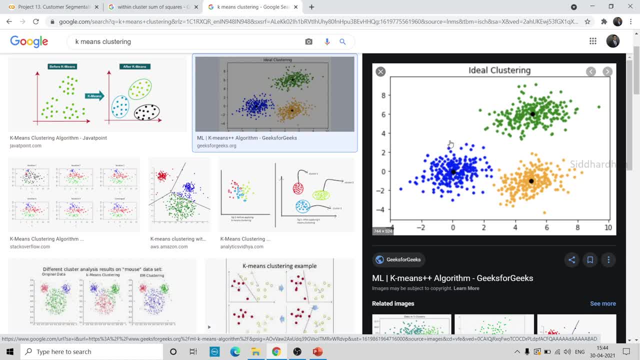 So these centroid are the representation point or the tresformation point. So these centroid are the representation point, presentation point or the midpoint of each cluster. So the midpoint or the centroid of this particular blue color clusters is this point, and for this yellow color cluster is here, it is given here the black one, and for it is also so each. 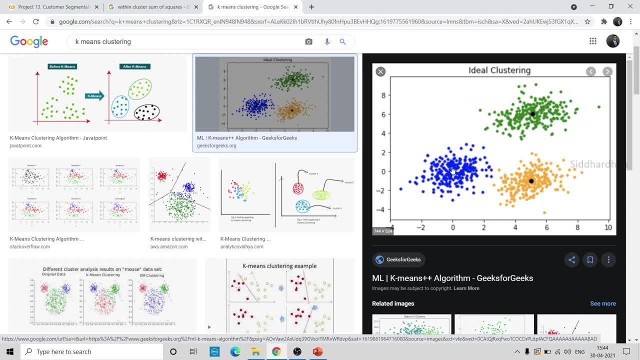 cluster as their centroid. So what happens is the K-means algorithm will randomly plot clusters. So in this case, the x-axis will be taken as the annual income. so, as I have already told you, so in our case the x-axis will be taken as annual income and the y-axis will be taken. 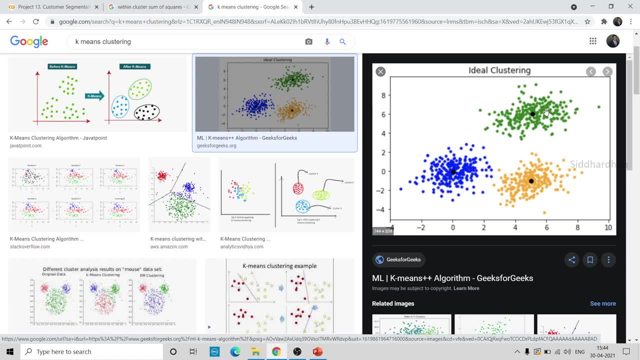 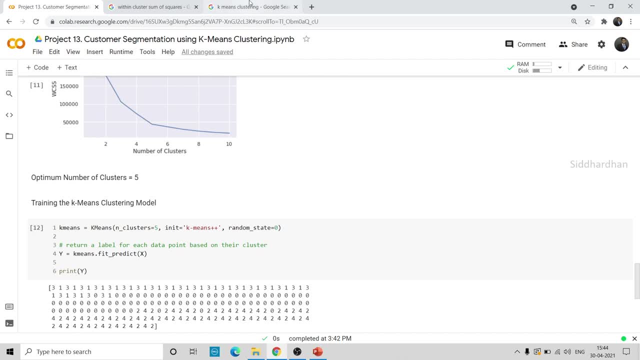 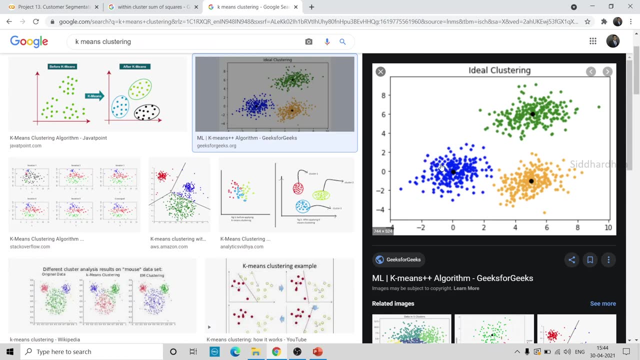 as their spending score and based on these values we will get different clusters. So in this case we have just only three clusters, but for this customer segmentation we got about five clusters right. so we will have five centroids and each data point will be plotted in this graph and their distance from that particular data point and this centroid. 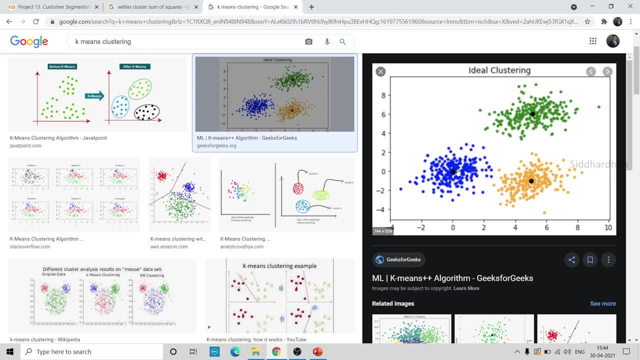 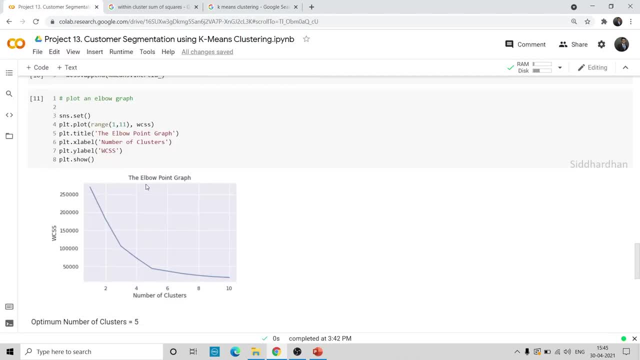 so each of the five centroid should be calculated and only one centroid will be closer to this value. Say, for example, we are taking this first value, okay, So the first value Is nothing but fifteen comma thirty nine, right? yeah, the annual income is fifteen thousand. 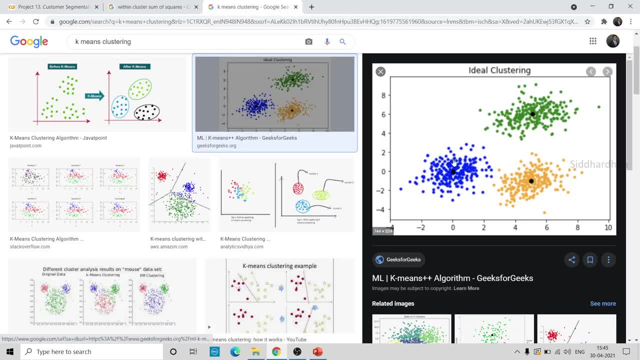 US dollars and the spending score is thirty nine. So we have randomly plotted five centroid values and it will be plotted in. those centroid values will be plotted in the graph and we will plot this fifteen comma thirty nine. So fifteen is the x-axis value, thirty nine is the y-axis value and it will be plotted. 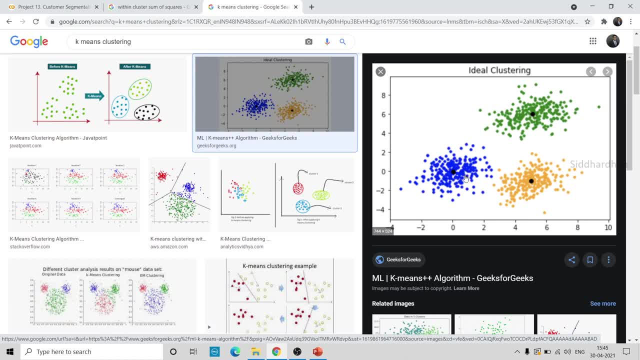 and the K-means clustering model will check which centroid is closer to this data point. So then the centroids will be moved accordingly. after all the data points are taken, All the data points are plotted, so when this process is completed, you will get different clusters and also their centroid as well. so the centroid are the very important thing. 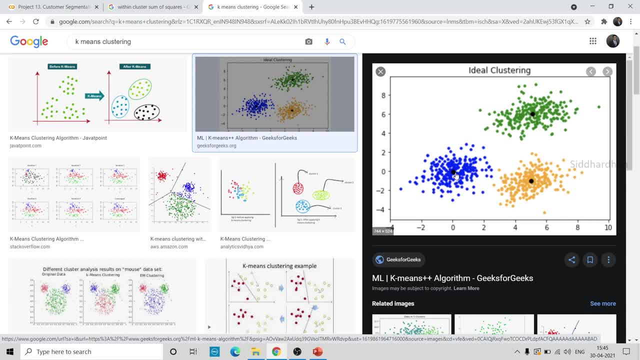 here so you can understand how this particular clustering works in the future. but just let us see how we can visualize this data. So this is the basic working of our K-means clustering work. so you just need to know that the centroid will be plotted first and then the data point will be plotted and it will 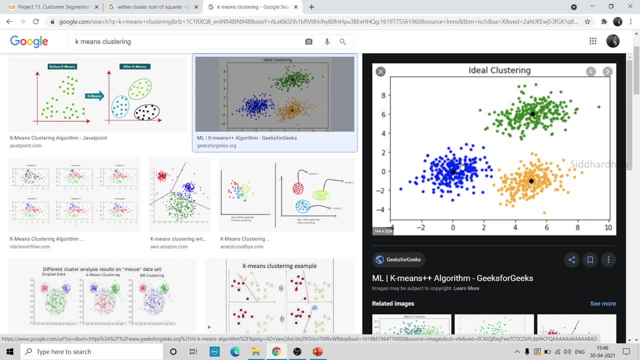 be checked that which centroid is closer to this data point. So the centroid is closer to that data point and then it will be rearranged. So this K-means clustering model will reiterate- I mean reiterate means it do this again and again to find the correct clusters that the data point belong to, and after that we can. 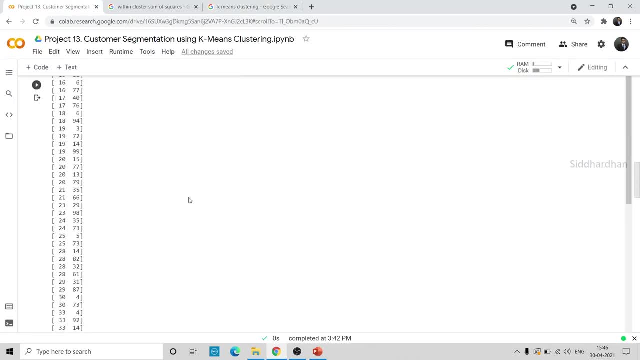 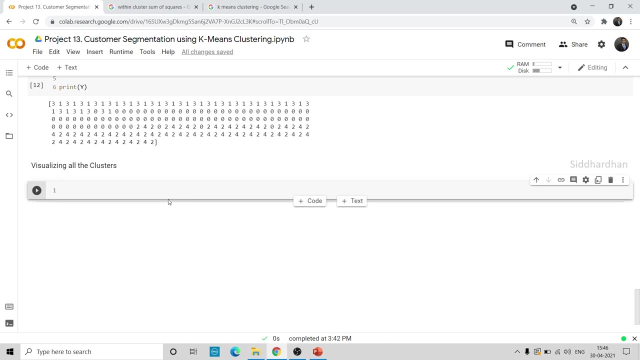 have clusters like this, so different clusters. So now let us try to visualize these clusters. so we just need to make some plots here, plotting all the clusters and their centroid. so centroid means the center point or the, you know, representation point of each cluster. so five clusters means we will have five centroids. so and their centroid. 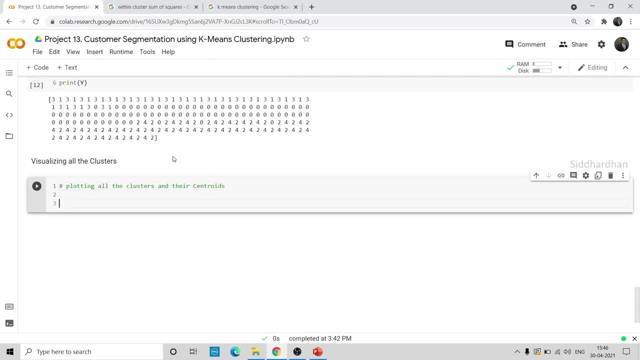 so I will show you how we can plot this. okay, so pltfigure. so we are creating a matplotlib plot and I will just mention the figure size here. so what is the size of the plot you want? and let us mention that 8 comma 8. so this is the x-axis unit and y-axis unit. so this is. 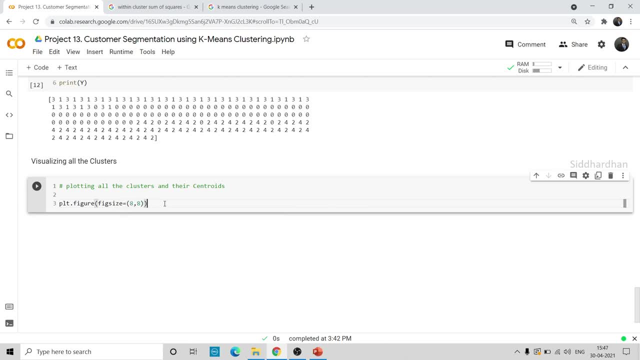 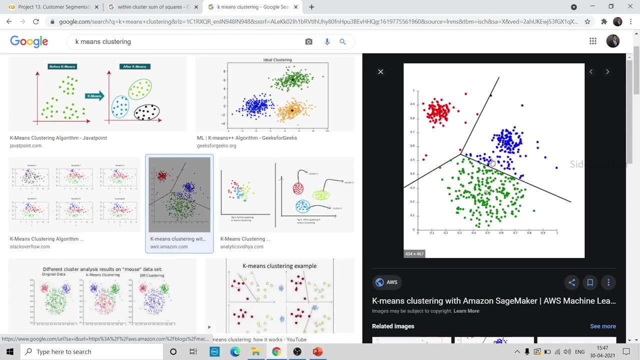 just for the size of the plot. so if you want a bigger plot, you can increase these values and pltscatter. so we are going to create plotters- sorry, scatter plot like this. so these are examples of scatter plot where we will mark different points. okay, so this is an example. 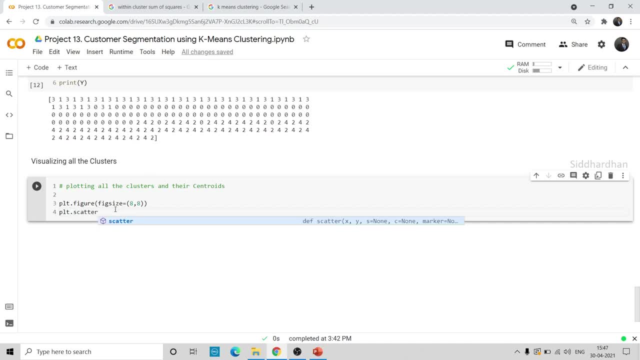 of scatter, plot, pltscatter, and so I just complete this code and explain you what I am doing here. So it is. it will make sense once I complete this. so y is equal to 0 comma 0 and x is nothing, but y is equal to 0 comma 1. s is equal to 50. do not worry, I will just mention you about. 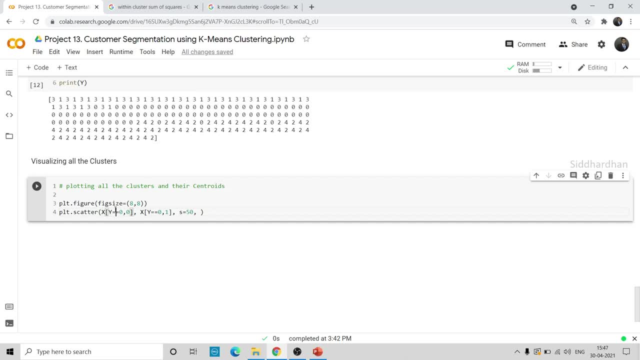 these parameters after I complete this line of code. this is equal to 50 and c is equal to green. Okay, c is equal to green. label is equal to cluster one. okay, so we just need to copy this line and paste it again five times, and we just need to change few things. 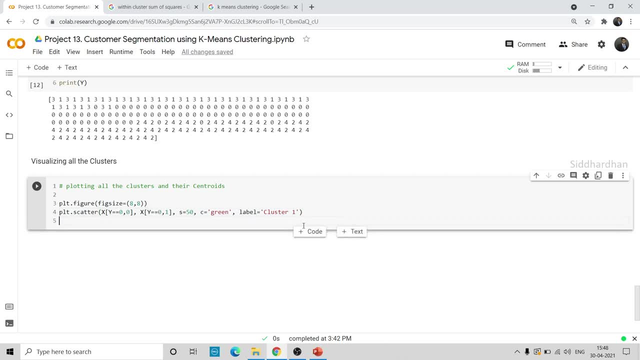 First is the x coordinate, y coordinate, size of the point. okay, so I will just put it five times. okay, so I will just change this cluster to cluster two, three, four and five. so totally we have five clusters and we need to change these values as well. so first one is 0 comma. 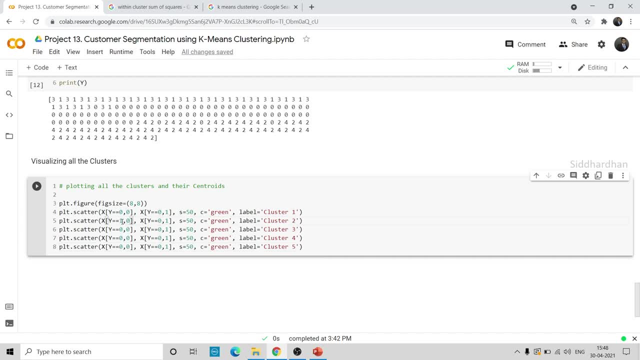 0, then we need to change this as 1 comma 0. I will explain you what these numbers signifies in a minute. So 2, 3 and 5.. Okay, And 4. and then here we have 0, 1, 2, 3 and finally we have 4. okay, so 0 comma 0. okay, so what we? 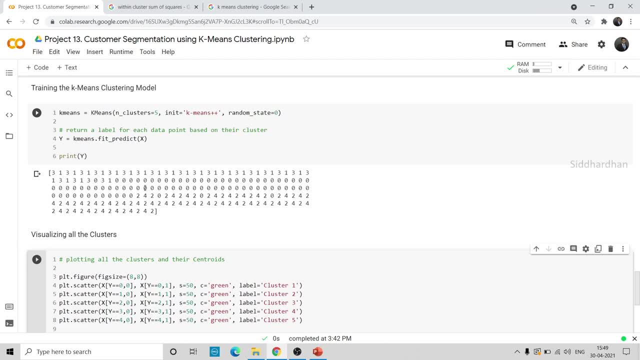 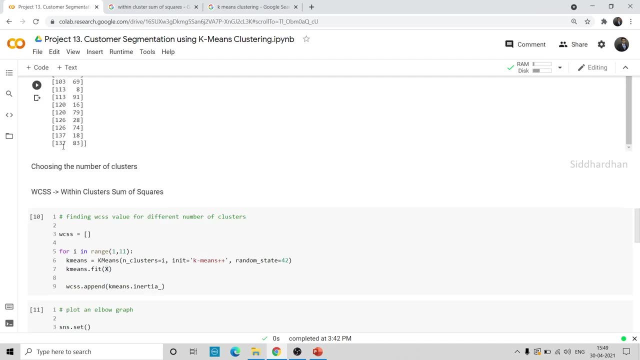 are doing is so this: all these y values. so y represents their cluster identity, or cluster label corresponds to this x. okay, so here we have this last data point as 137, comma 83, and the label for this last data point is this last value, which is 2.. 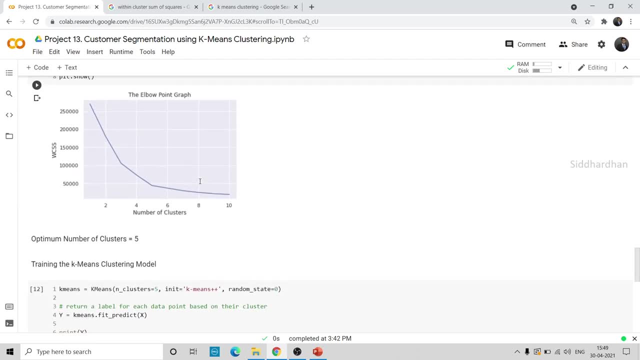 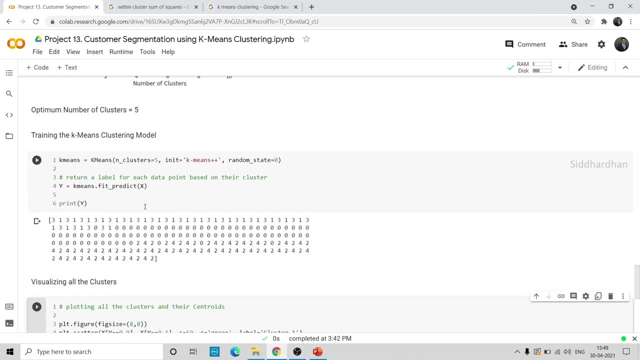 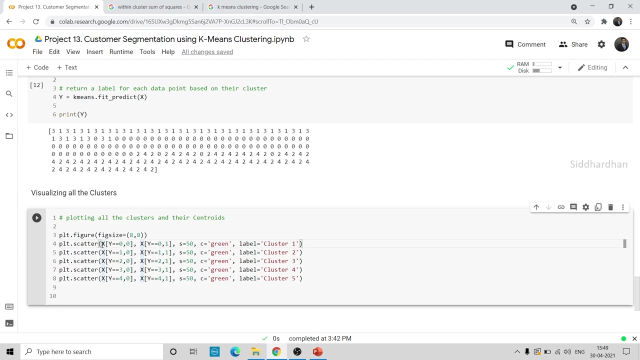 So that means this particular value belongs to second cluster, right? so this second cluster. so we need to plot this data along with their clusters. so here we have this: 0 comma 0, so this particular point here. so from this, sorry, so from. so this is the x coordinate of this. 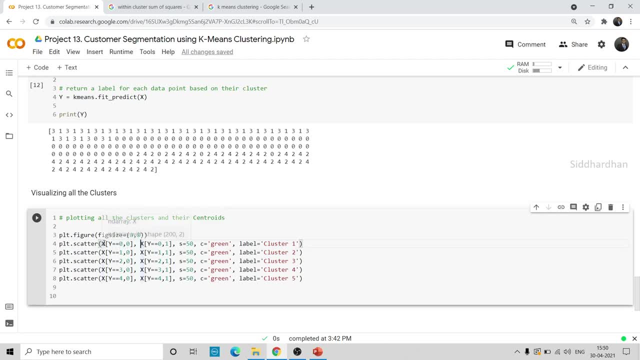 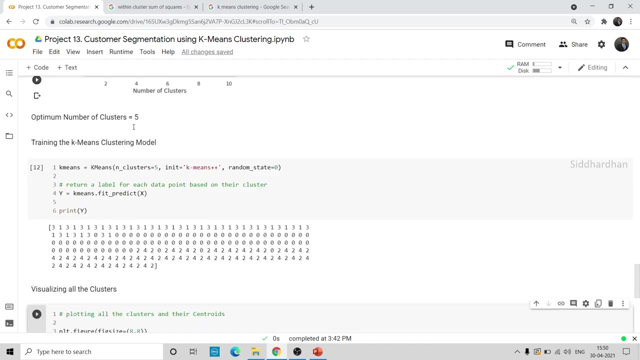 particular cluster one. Okay, So for here we have x, and y is equal to 0 comma 0. so this is the x coordinate and this is the y coordinate. okay, so for all the clusters one and cluster one is nothing but the label is 0, right? so totally, we have five clusters here. here the five clusters are nothing but. 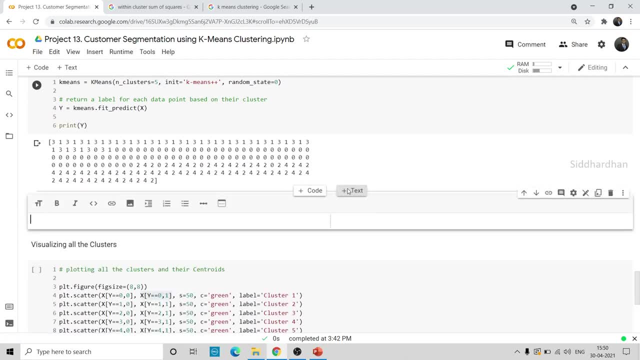 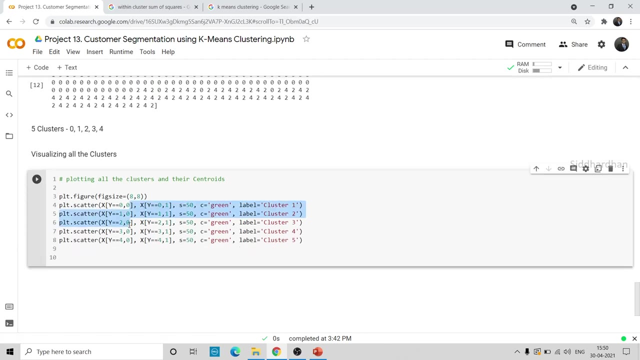 I will just put a text here so it is better for your understanding: five clusters and each of the clusters as. So the five clusters are 0, 1. 2, 3 and 4. right, so here? the second value here represents the first cluster. so I want. 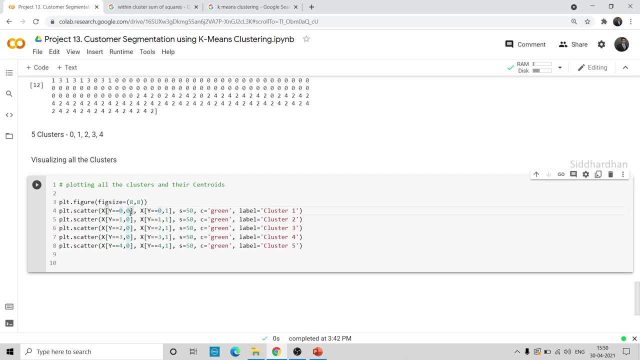 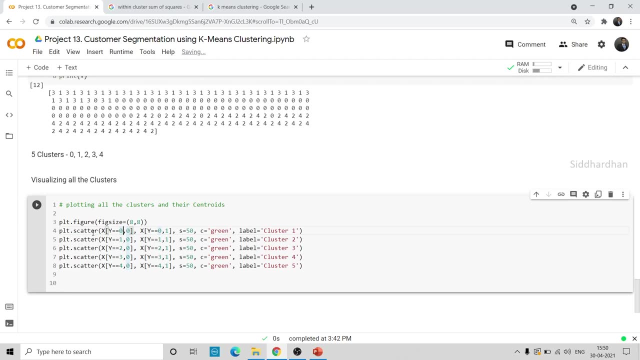 to plot all the first cluster value, and sorry. okay, so this is the. so I here I have mentioned 0 comma 0. here the 0 represents the cluster number. so that means I am plotting the first cluster. so you can also see here that I have mentioned cluster 1, right? so when I mention: 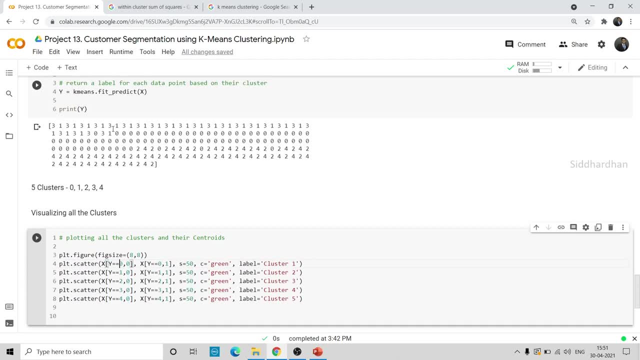 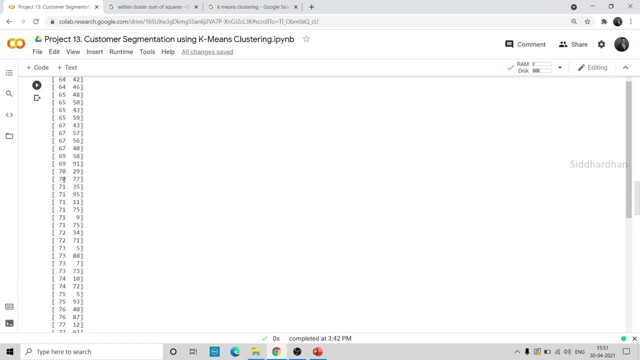 0. here It will take All the values Of Cluster 0, or that means the first cluster, and here we have the second 0 right. second 0 represents the first column of this x. so the first column is nothing but the annual. 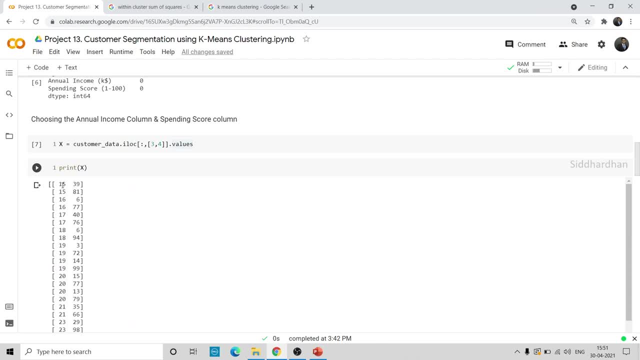 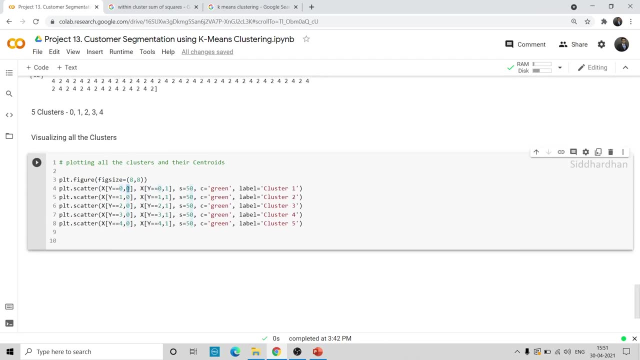 income and the second column is spending score. so the index of this first column is 0 and the index of the second column is 1. so that is what we have mentioned here as so you can see, here all the values are 0. so here the x coordinate is taken as annual income, because 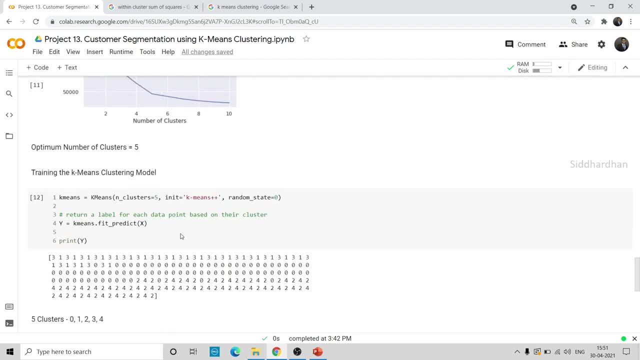 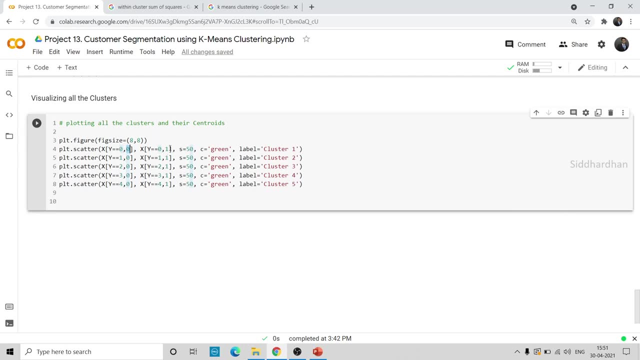 we know that the 0 represents the first column, which is annual income, So we have mentioned all of them as 0 and all of this first part represents x axis and the second part represents y axis, and all the 1 represents the spending score, which 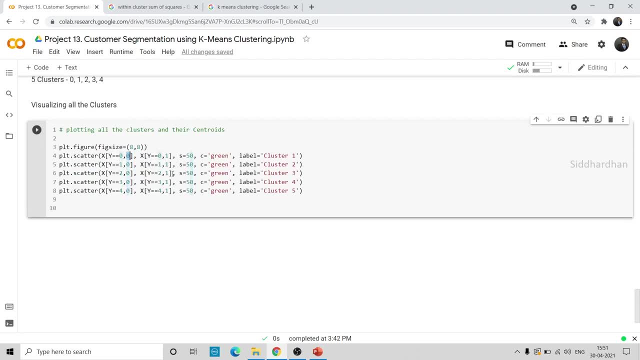 is the second column value. so I am just giving x axis and y axis value and the first line is for first cluster. so that's why I mentioned 0 in the first value here. 0 here and 0 here represents the first cluster. right now it will change, so 1 means the second cluster. 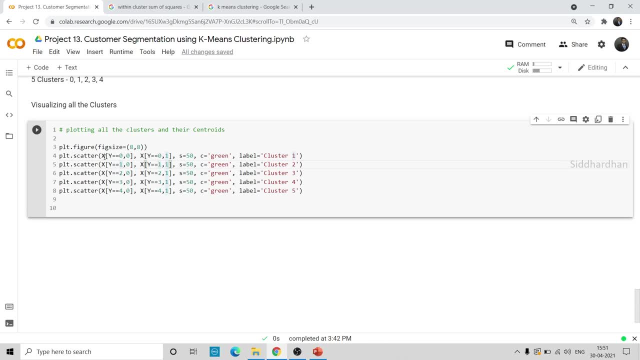 here we also have 1, again 2, 3, so we have 5 clusters. so each of this represents data point of each 5 clusters. and here the 0 represents the x axis value, which is annual income, and here the 1 represents spending score. so this will give us a data visualization and plots. 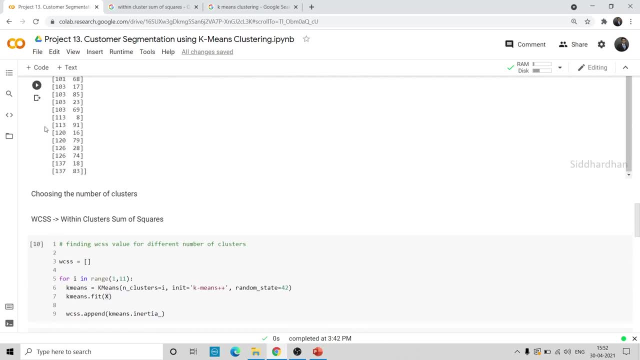 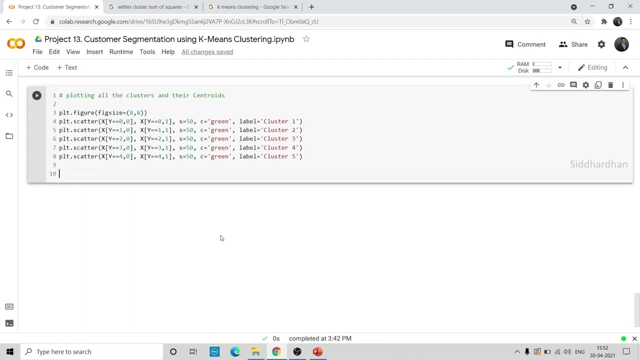 of all the data points, along with their annual income and spending scores, as well as their labels of clusters. now we need to plot the centroids, as I have mentioned you. we have this centroids right, so this black dots, so those are almost the center point of each clusters. 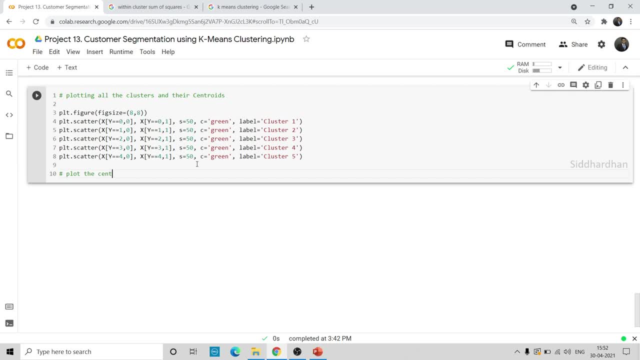 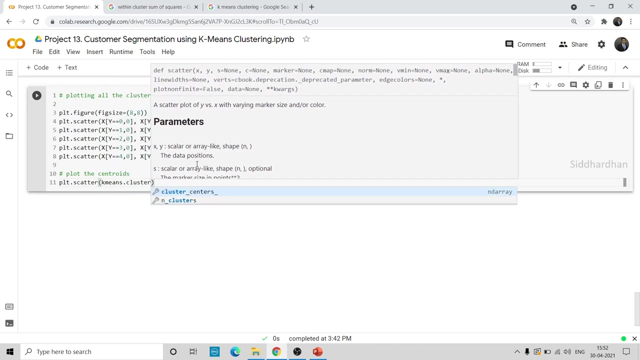 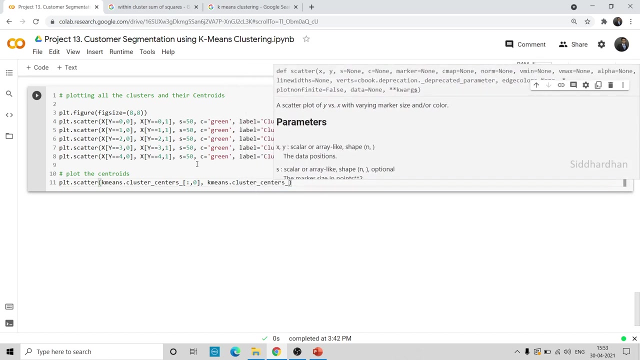 Now we are going to plot the centroids. ok, so plt dot scatter kmeans. so kmeans is the function which we have loaded. kmeans dot cluster, cluster center. so this is the centroid values. so we need to mention colon comma 0.. And kmeans dot cluster centers 1. ok, so it is very similar to the one which we have did before. 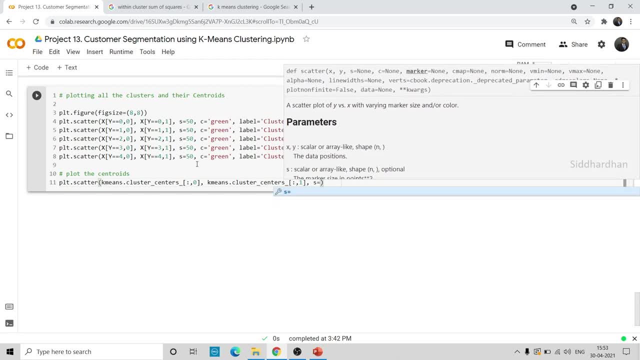 I will explain you what we are doing here in a minute. s is equal to 100 and color is equal to, which gives 7, so it looks different. And here the label is 0.. And here the label is 0.. And here the label is 0.. 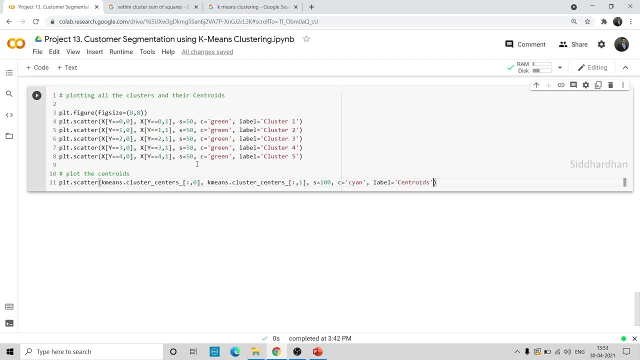 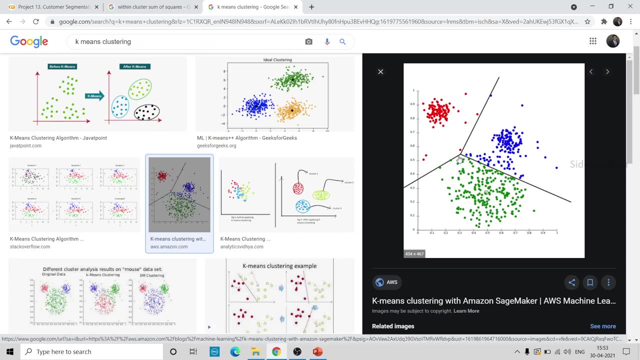 So here s represents the size of the dots. so I have told you that we are going to make scatter plots, right? so Scatter plots, we should make these dots and we need to mention the size of this dots. so if you increase this size, you will get bigger dots. and the c represents: 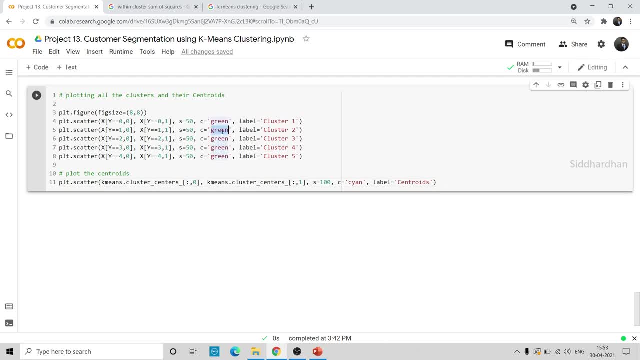 the color of the dots. we can give a different colors here, so I will just change colors to red, put each cluster in a different colors. so green, red and we can take yellow color in this. so just take five different colors. so c represents color and we need to give those parameters and blue. 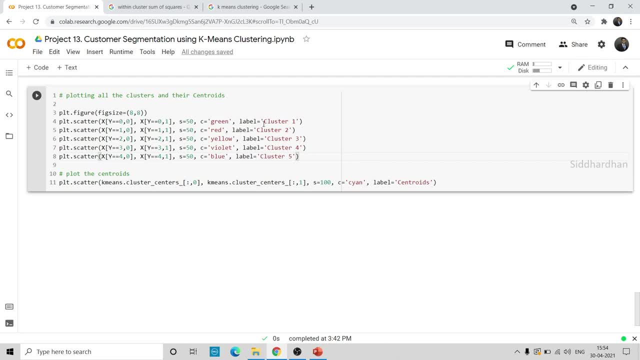 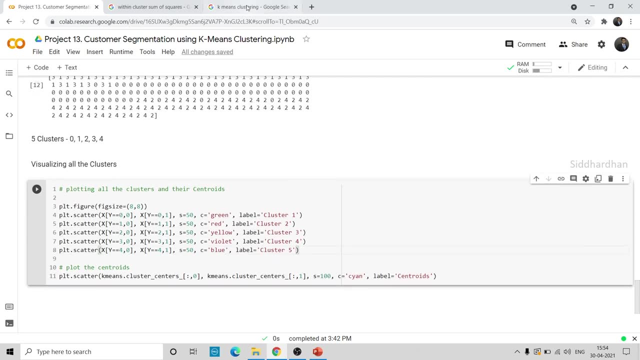 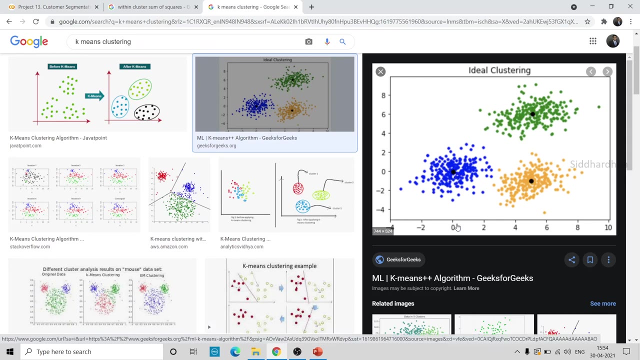 so each cluster will look in a different color. okay, and finally, we have this centroid values. here, zero represents the centroid of those exact. so you know when you have a plot. so let's take this: when you, you know, choose a particular dot in a graph, we need x-axis as well as y-axis, right? 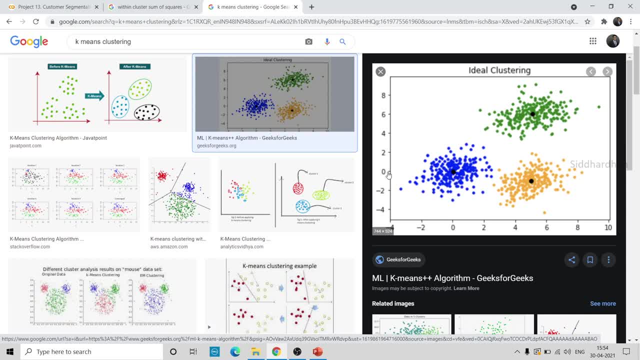 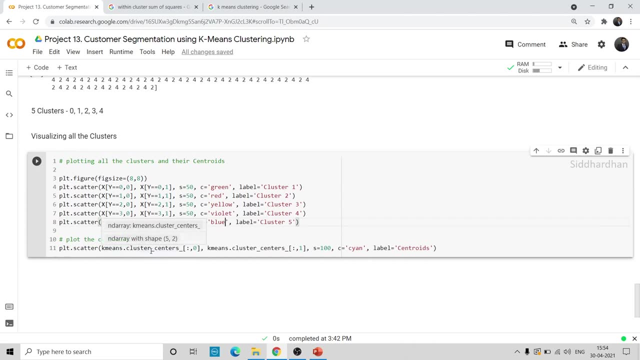 so for this particular centroid the x-axis value is zero and y-axis value is also zero, so for this it can be around five and almost it's minus one, right? so we need the x-axis value and y-axis value for any point to mention here. this zero represents the x-axis value of clusters, sorry. 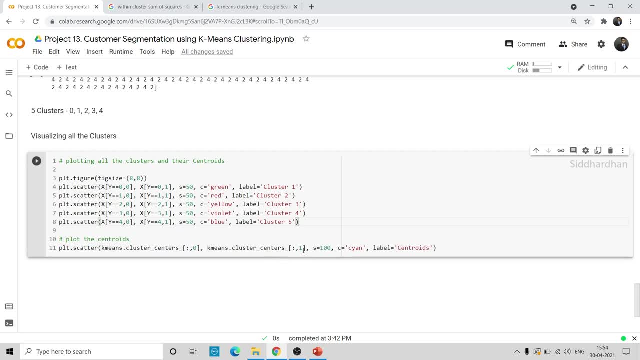 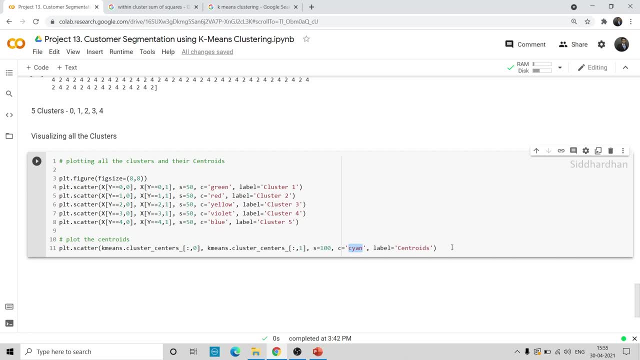 we are taking five different colors for all the centroids. now we can just give the names for our plots and plot this graph. so i'll give the title as plt dot title. let's name this as customer groups. okay, you can just mention it groups or clusters, anything you want. i'll just mention this as. 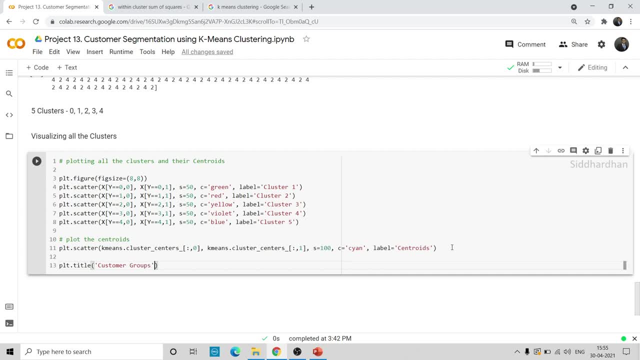 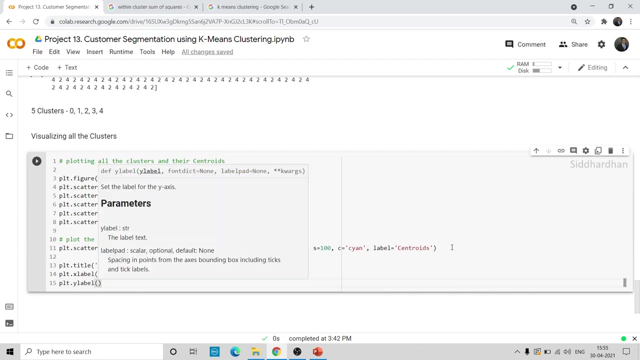 customer groups and plt dot x label: annual income. so we are taking annual income as our x-axis and y-axis will be spending score, right. plt dot y label: it will be spending score, so the spending score value ranges from one to hundred spending score. we can finally use plt dot show to print our graph. let's see whether we did all the things. 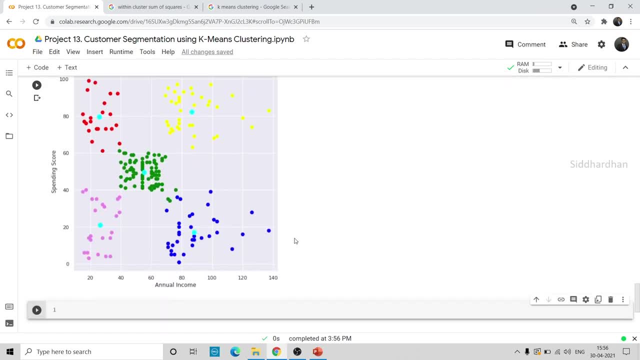 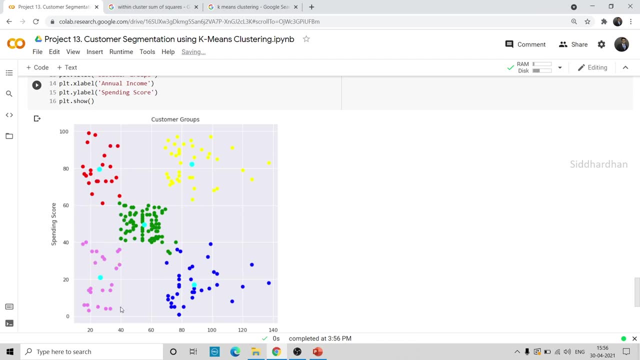 correctly. okay, so this is our plot. so, as you can see here, we have multiple clusters here. so this is one cluster, there's red in color and we have a violet color cluster, green color cluster, yellow and blue. so you know, all these clusters are, uh, partitions in, partitioned in a good way. 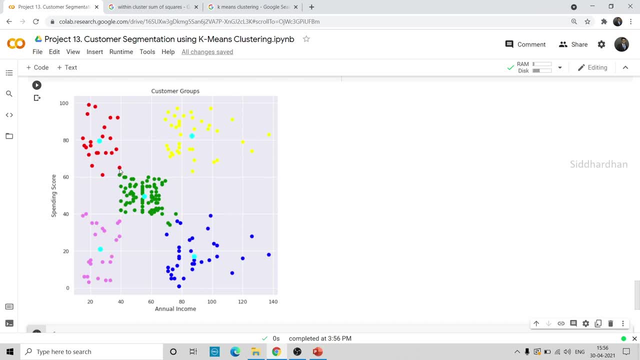 there is not any mix. so here we have just close values between this data point and this data point, and this one and a few data points are closer to each other and apart from that, all the clusters are, you know, partitioned in a different way. so this is the clusters group of customers which we 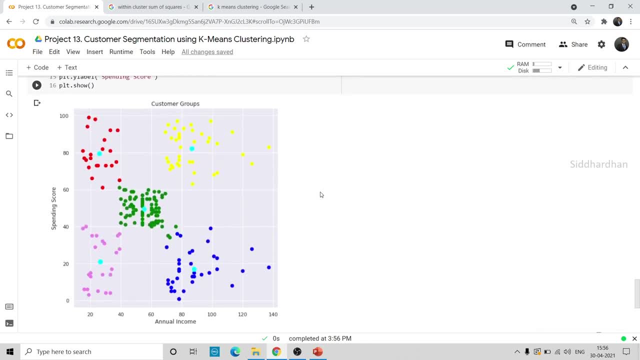 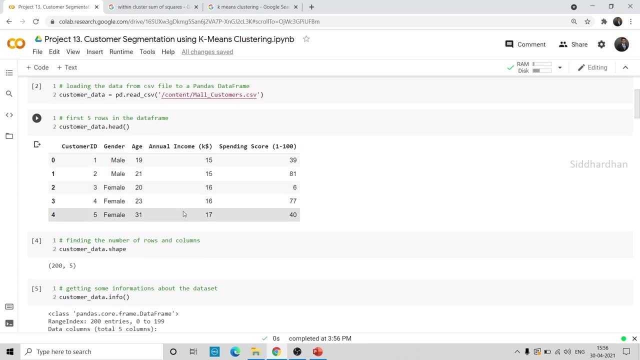 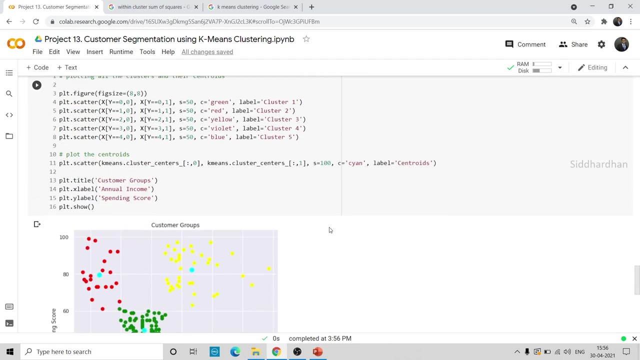 are getting. so this is an amazing data visualization to see that our data points- sorry, our data set as so we are. so this is the data set as five different groups of customers, so let's just get some insights from this, uh, particular visualization. so here, red color is the second. 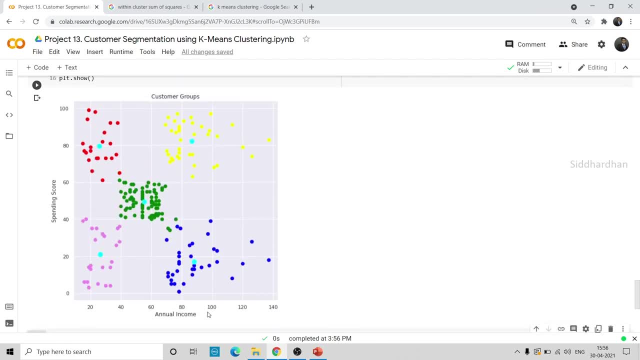 cluster, right? so just look at this graph. so in the x-axis we have annual income and in the y-axis we are spending scores. so if you take this particular red color group of people, so this is one cluster and this particular group of people don't have a very high annual income, but they have a very good. 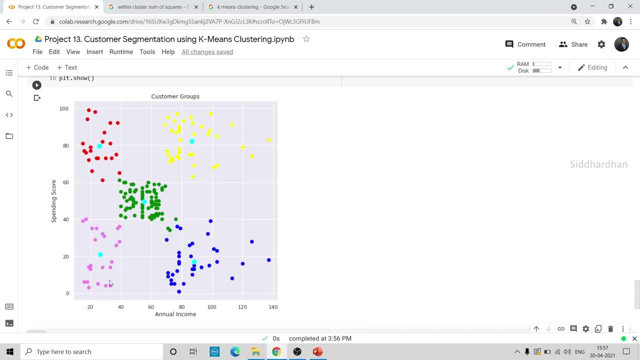 spending scores. but here, you can see here these people, these group of customers, has a very less annual income and also they have a very less spending score, which is like understandable because, like, people with less income tend to purchase less in supermarkets and malls. and you can see here this, this particular set of people, as you know, kind of more annual income but they 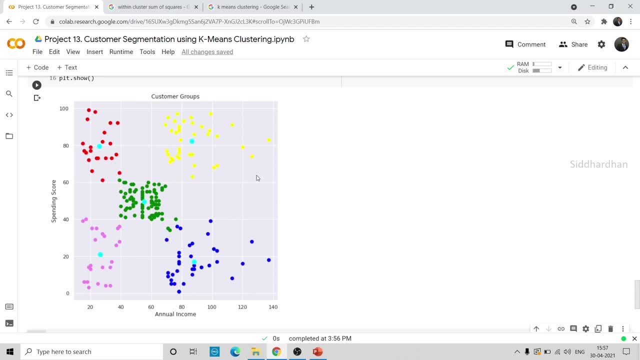 don't spend much, so they are just cautious about what they are buying. so this group of people represents people with more annual income, and they are spending a lot right? so these are the insights that we get. so what this mall can do is they can give offers for those people who are just not. 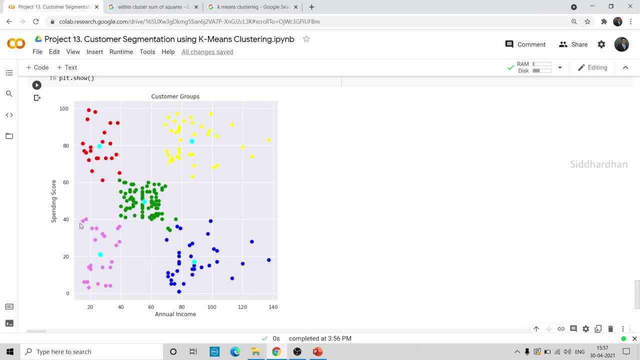 buying too much. So here we can say that people who are not spending that much. so we know who these customers are and we can give better discounts and offers for these people using some membership cards. and we also can give offers for these people who have high income value and also have very less spending in. 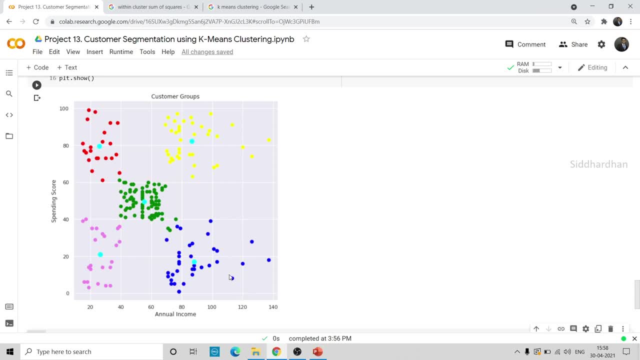 that particular mall. so when you give more offers and discounts, they can tend to- I mean they tend to buy more right. so this will increase the profit of that particular mall and it will increase the customer satisfaction. So this is how the malls can improve their income. 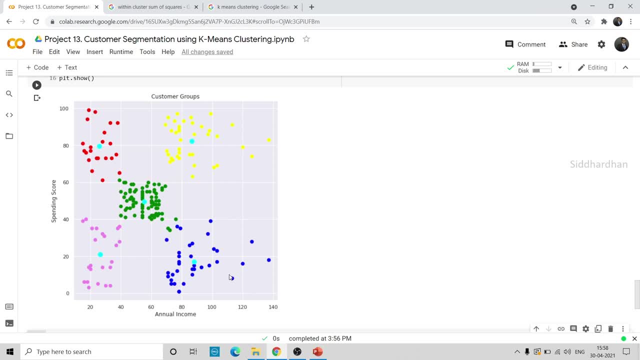 So that this is how the malls can improve their- you know- market value and then improve their profits. So this is the very important business insight that we get from this clustering. So this is how you can take a data set and you can find some clusters or groups of people and can 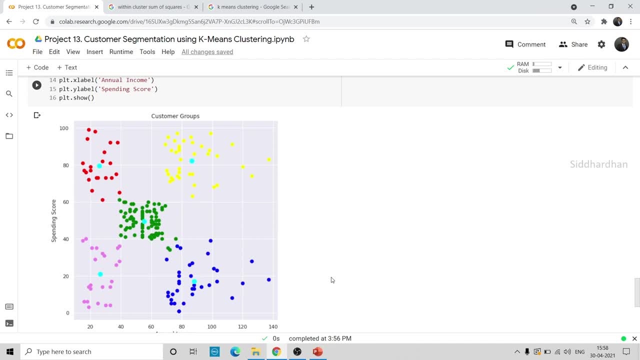 make better recommendations for them. so there are a lot of applications for this clustering. I would like to give you a few more examples. let's say that there is a movie watching platform like Netflix or Amazon Prime, So group of people who tend to watch thriller movies or horror movies. when a new person 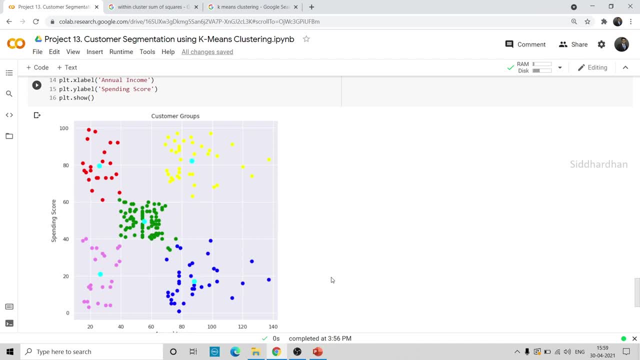 watches a superhero movie. this netflix system can suggest the movies based on the group of customers or big, you know, group of people who are watching superhero movies like. so by this method they can give better recommendations for people. so, similarly, uh, google ads and other things work where they. 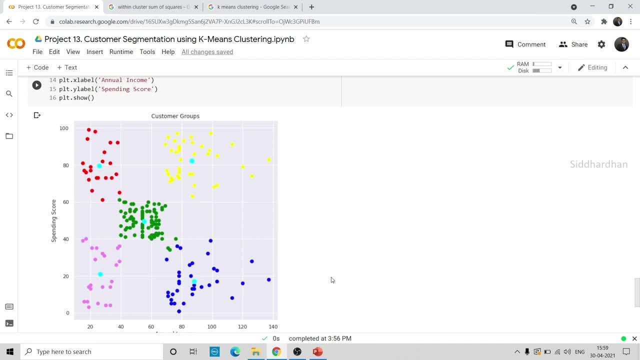 group people in, you know, based on their different interest and using this data, they can make better recommendations for them. so there are a lot of applications that can be done using this clusters, so you can just search for them. on what are the different aspects that we can do: